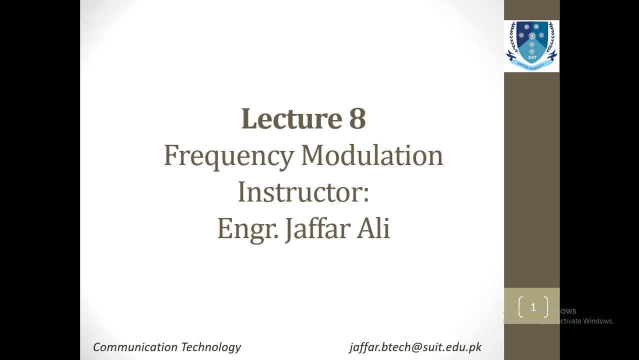 in mind, we are heading towards our next topic, that is, frequency modulation. So today's brief, today's lecture briefs, is shown to you now, Now on the screen. so the topic that we will be covering in today's class will be the frequency. 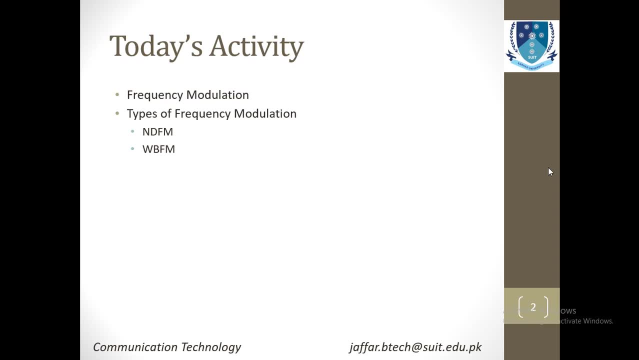 modulation. that? what is frequency modulation? how does it actually work? the operation, the phenomena, the considerations, the parameters, the all of the features, the advantages, the disadvantages, all these things will be discussed in today's class, along with their two types, The. 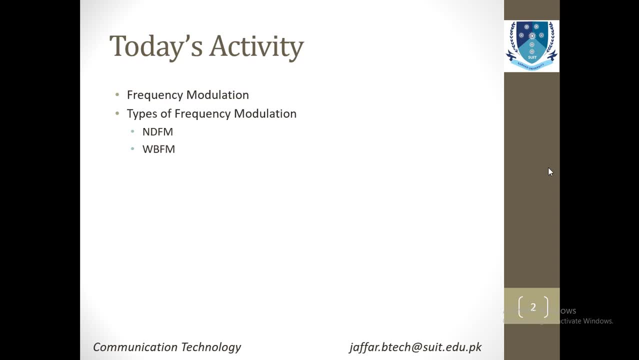 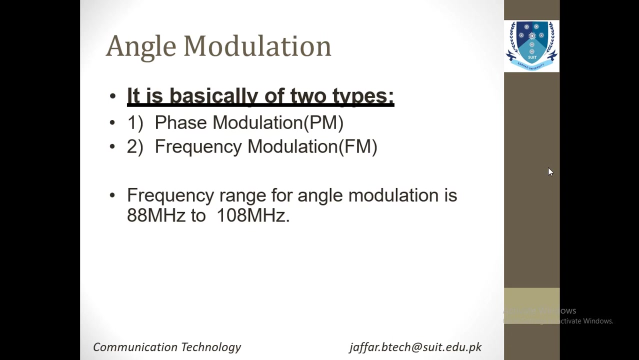 first one is NBFM, that is, narrow band frequency modulation, and the second one is WBFM, that is wide band frequency modulation. So we will be discussing these two classes, as well of these frequency modulation, into this lecture. so stay hold. So we have already discussed that there are two subclasses or two subcategories of angle. 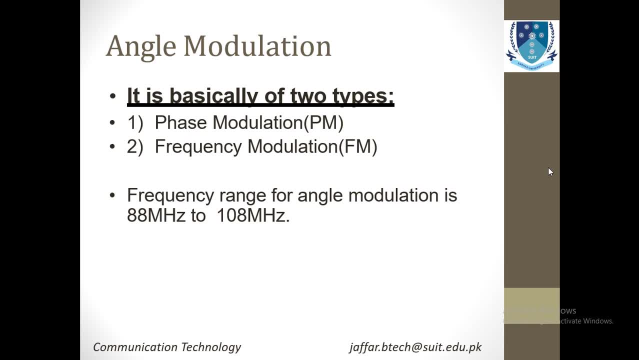 modulation. The first one is known as frequency modulation and the second one is known as phase modulation. So these are two. basically are the subclasses, and I have also already also asked you one question, that why do we categorize both of these? Why do we categorize both of these? 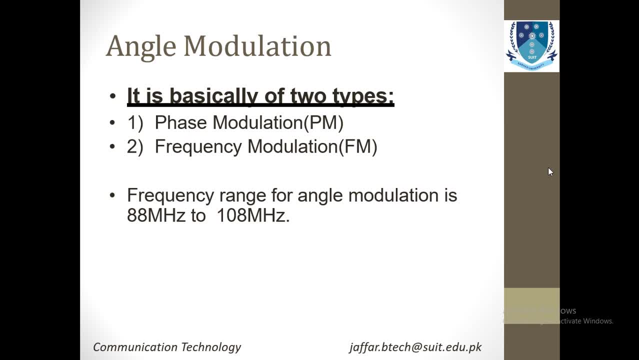 Why do we categorize both of these Modulation techniques, that is, frequency modulation and phase modulation, into one class, that is of angle modulation? Why do we keep these two- and why not? amplitude modulation is over here- Why these two are classified in this one single class of angle modulation. 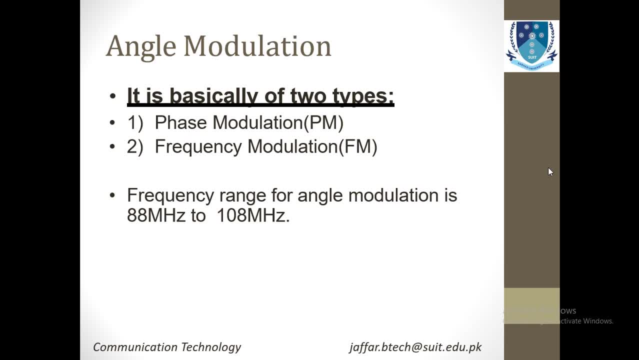 So this question still remains unanswered till now, and I hope that some of one of you- or some of you might be- have any answer for that. I will be waiting for that answer because you know that I have already told you that this question has three marks of its own, So you have to gain these three marks, and the time was before midterm. Anyhow, we will be focusing on frequency modulation in today's class. 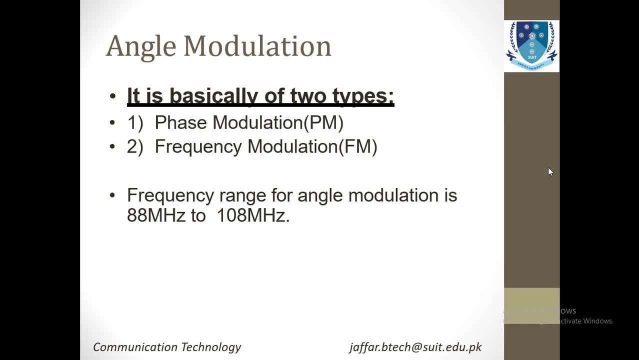 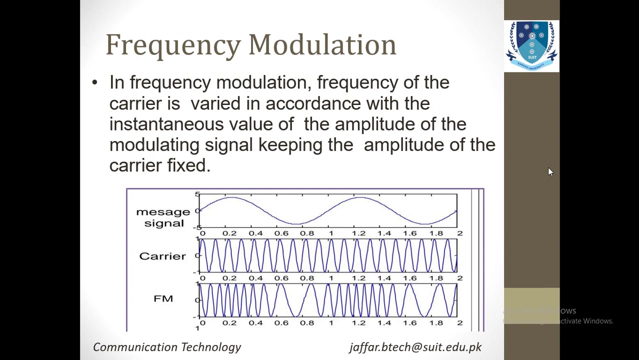 So the frequency range for the angle modulation varies from 88 MHz to 108 MHz. So this is specified for the angle modulation, not just frequency modulation. This frequency range is specified for both phase modulation as well as frequency modulation. Now coming towards our topic that is under consideration today, that is, frequency modulation. 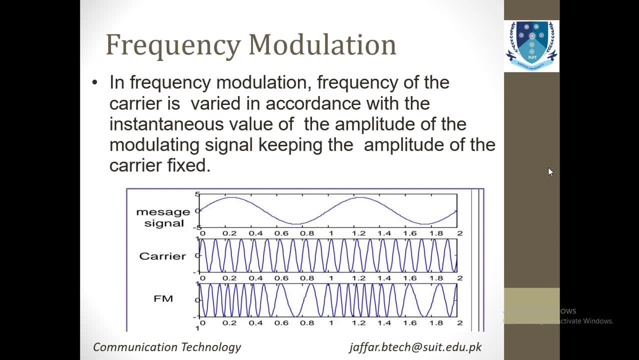 So I will also upload some theories- The theoretical portion and derivation portion- in the notes section that you will be having on the portal. So just to explain you in a very simple term, frequency modulation is that type of modulation in which the carrier is valid in accordance with the instantaneous value of the amplitude of the modulating signal, keeping the amplitude of the carrier fixed. 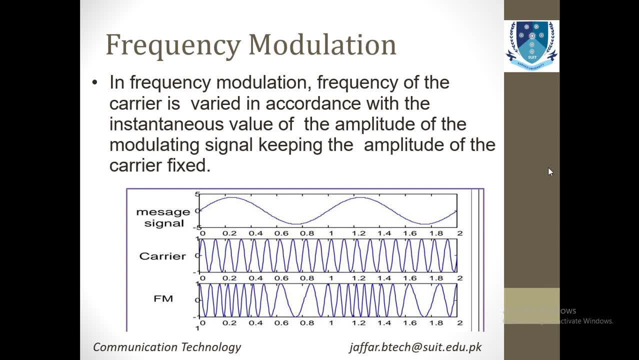 So your amplitude will be fixed. You will be only varying the frequency Of the carrier signal with respect to the amplitude of the input signal or your baseband signal or your modulating signal. So, based upon your amplitude of your input signal or your modulating signal or your baseband signal, you will be varying the frequency of the carrier, not the amplitude, not the phase. 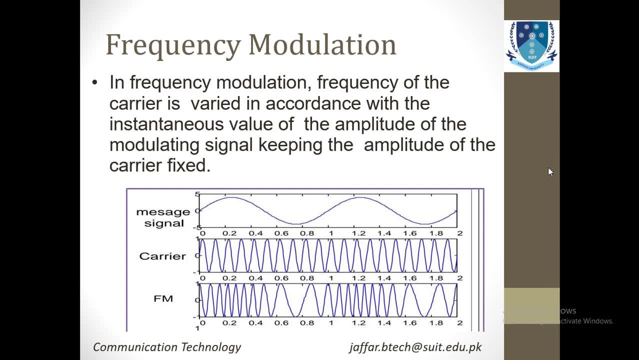 You will just vary the frequency of the carrier, and this is known as angle modulation. as simple as that. I have shown you a diagram. In the figure you can see that the message signal has two peaks: amplitude. the first one is plus five and the second one is less than minus five. 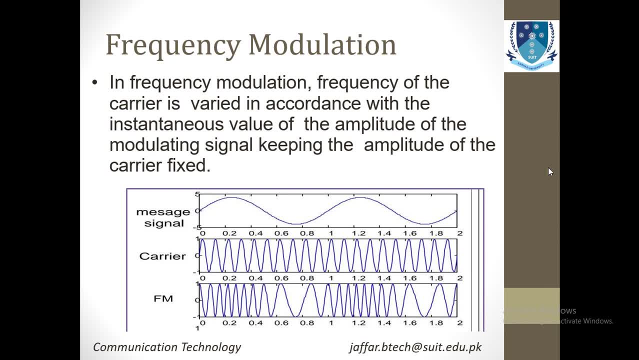 So you see that and the carrier is the same for all of these and the FM generated wave that we have generated the modulated signal. you can see that whenever the amplitude of the message signal is high, the frequency is high, and whenever the mass amplitude of the message signal is low, that is minus five. 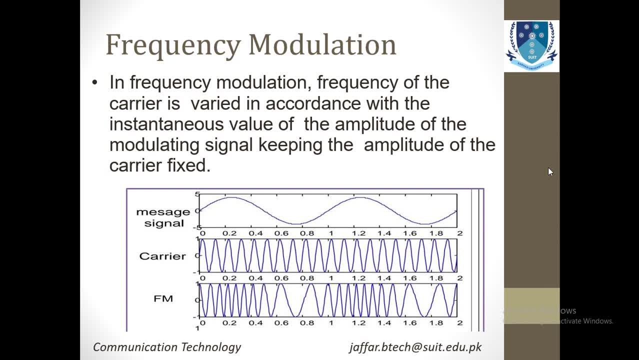 The frequency generated, The modulated signal, or the frequency of the modulated signal, is very low. You can see that. Let me show you. You can see that when this frequency is, this, amplitude is five at this point from here to here. So the amplitude will be high. 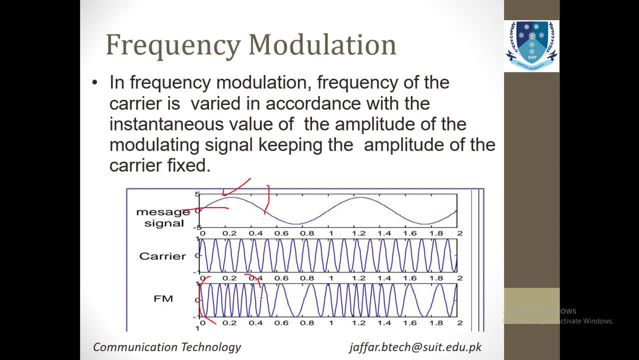 You can see that the amplitude, The frequency, is high And when the amplitude is low from here to here, And when the amplitude is low from here to here, You can see that the frequency of the modulated signal is very much low. So this frequency change is due to the amplitude of the message signal. 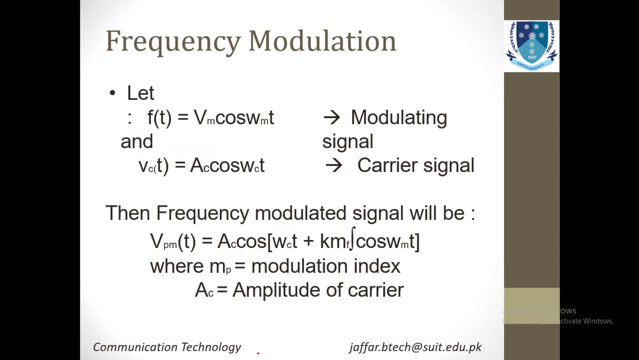 So this is known as frequency modulation. Let's talk about some of the mathematical portion, the derivational portion. I have given you this complete form of this And the complete derivation will be available to you on the notes. So let's consider that this f of t is basically your modulating signal or your baseband signal. 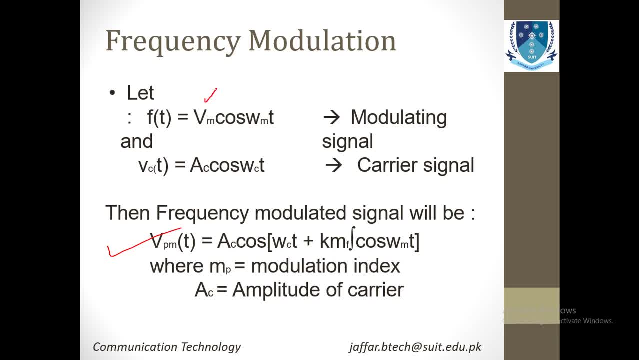 In which this vm of t, vm is basically your message signal And this is the frequency or angular frequency of your message signal, or your modulating signal. And this vc of t is basically the voltage of your audio signal, of your amplitude of your, the complete signal, of your carrier signal. 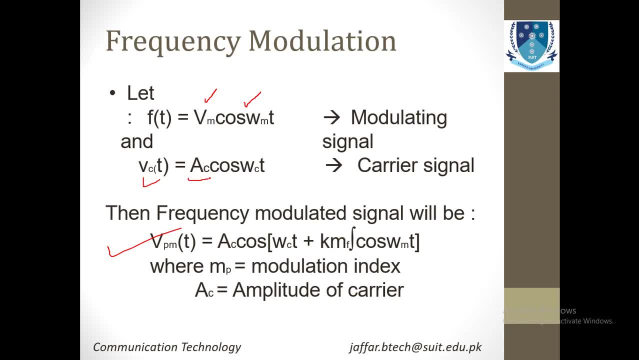 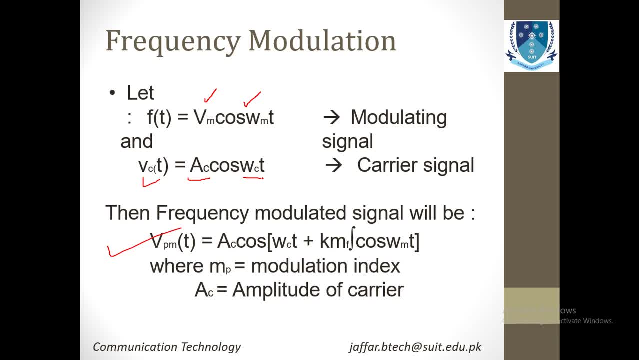 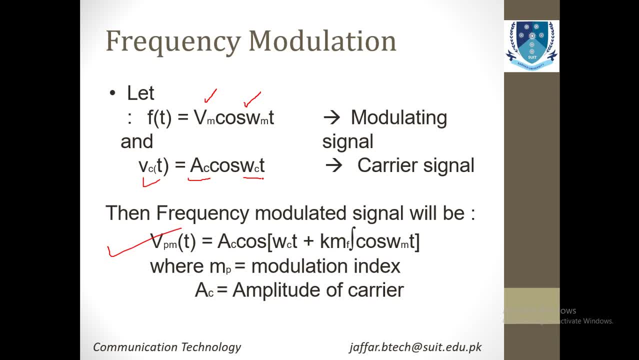 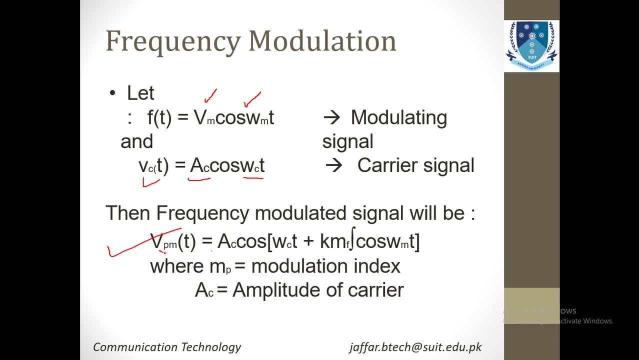 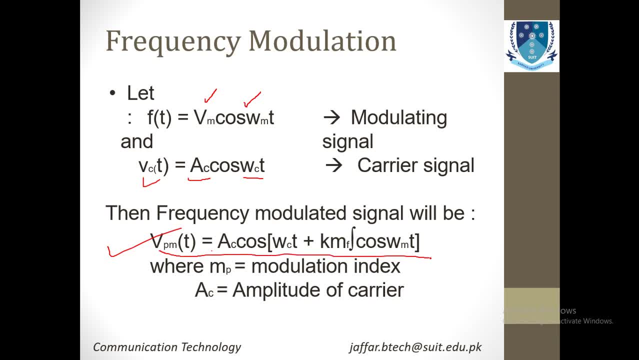 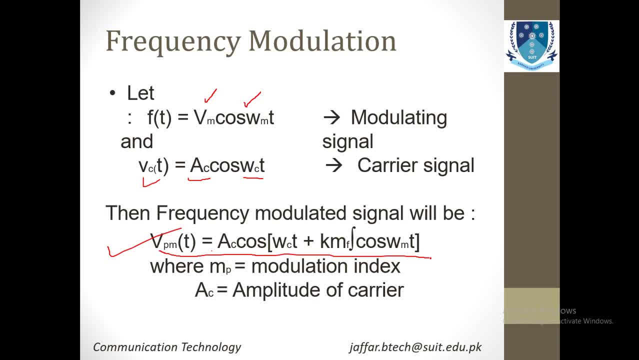 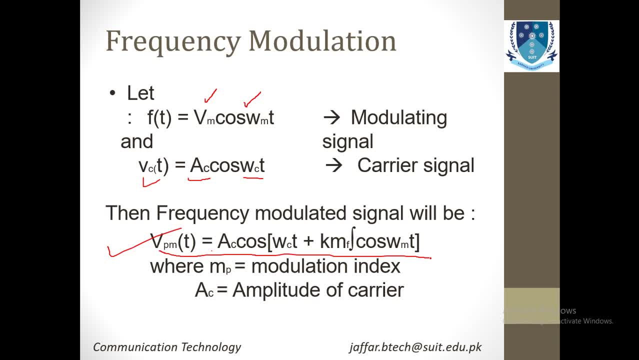 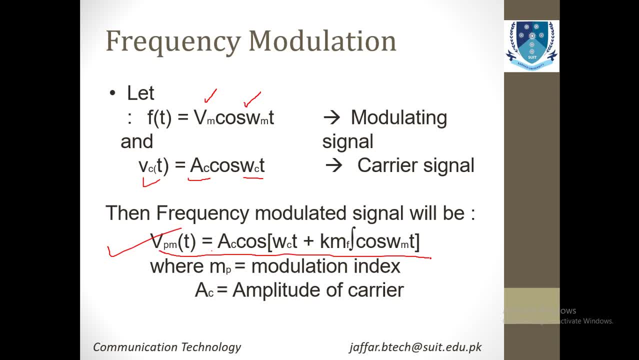 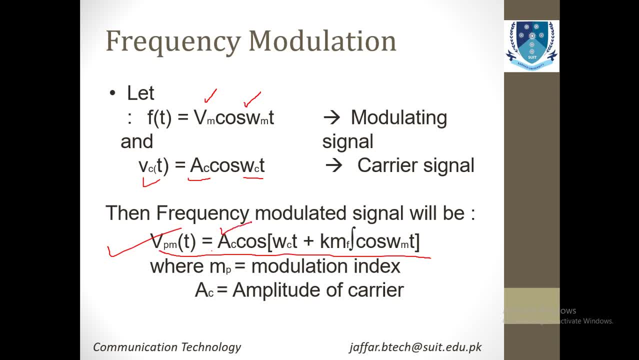 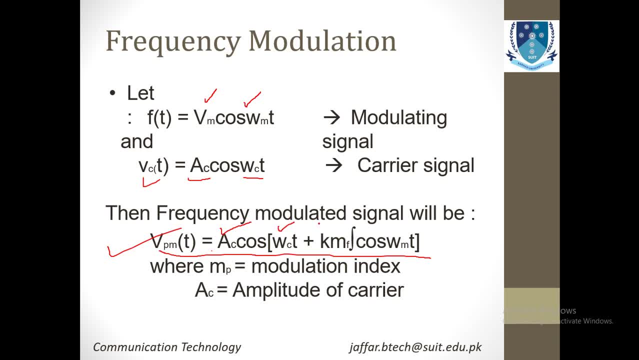 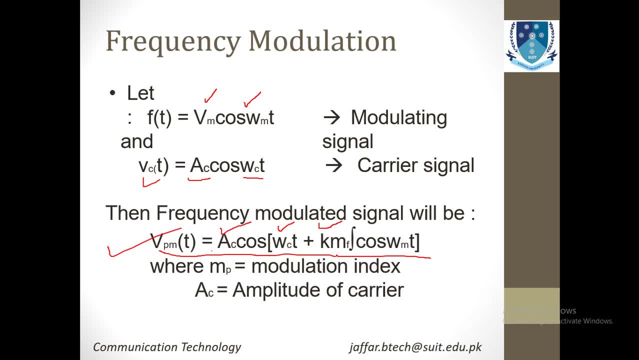 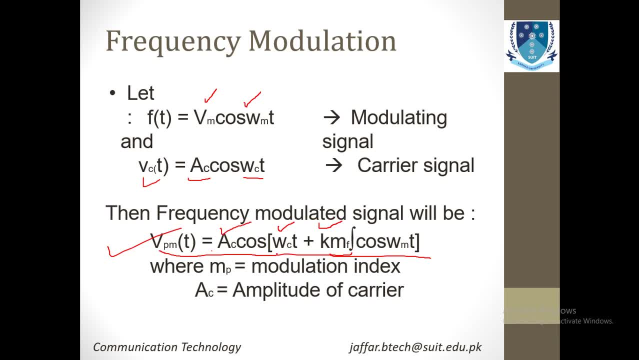 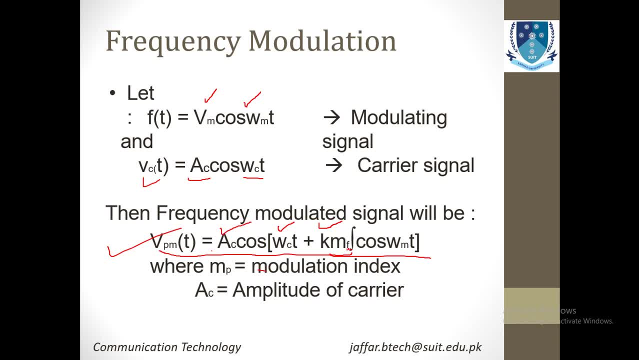 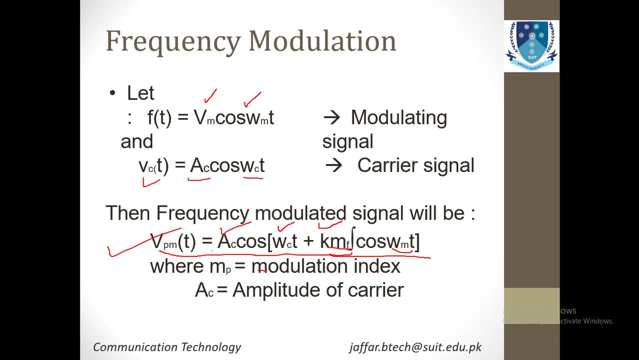 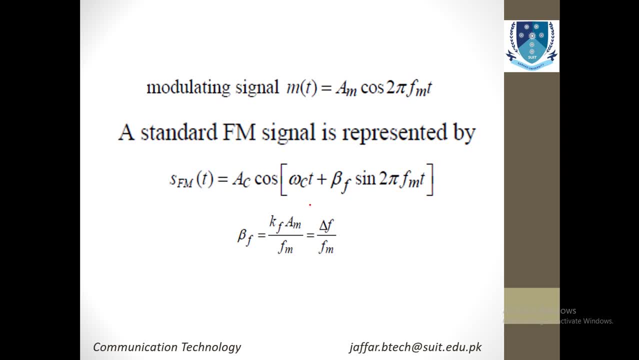 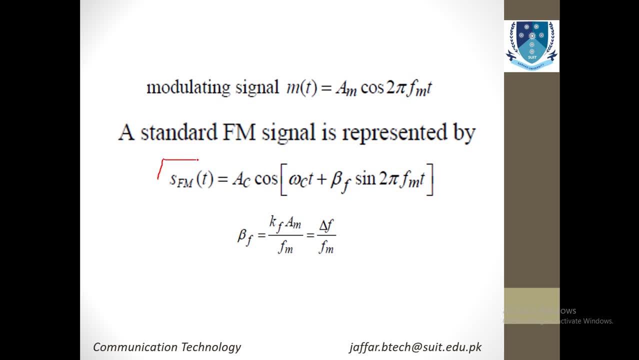 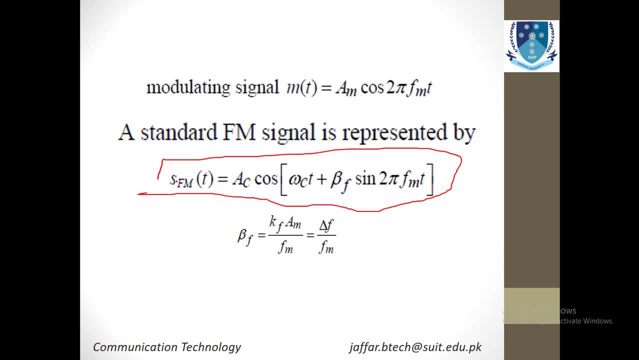 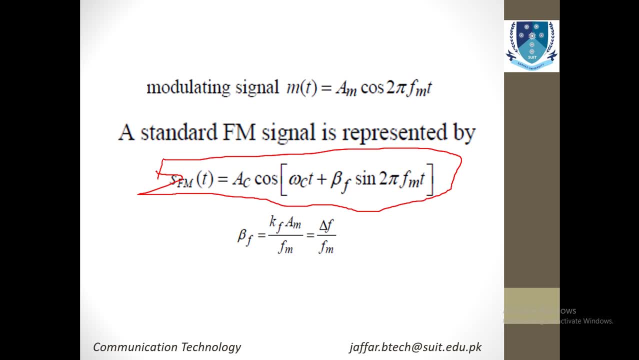 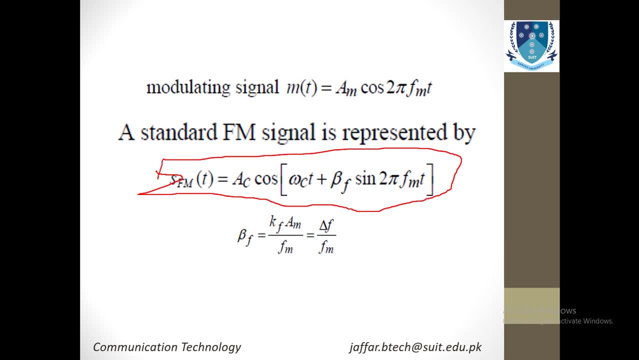 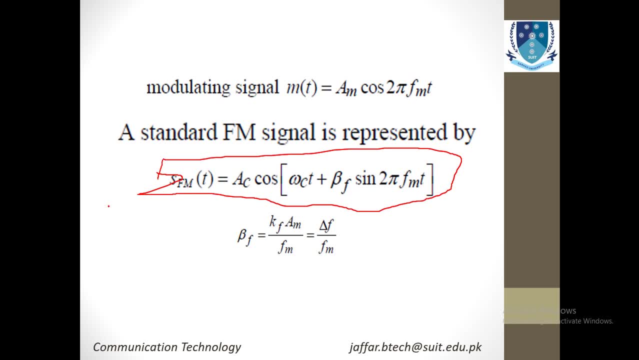 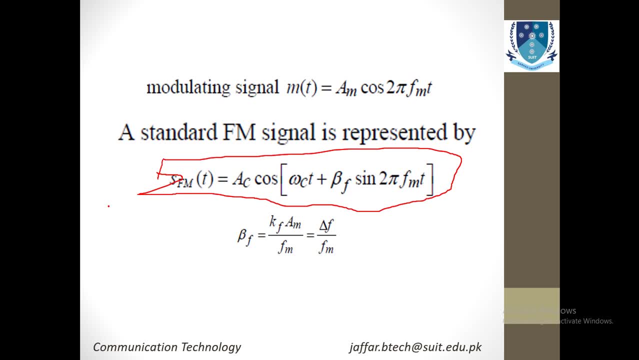 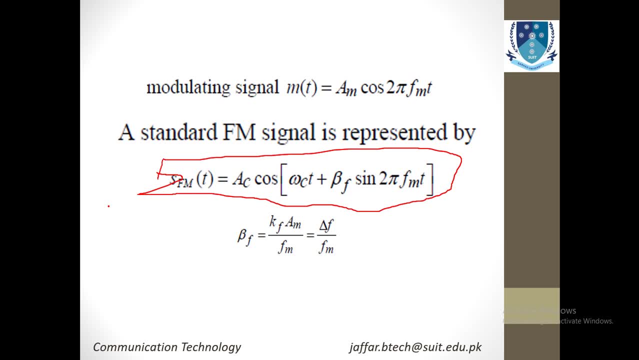 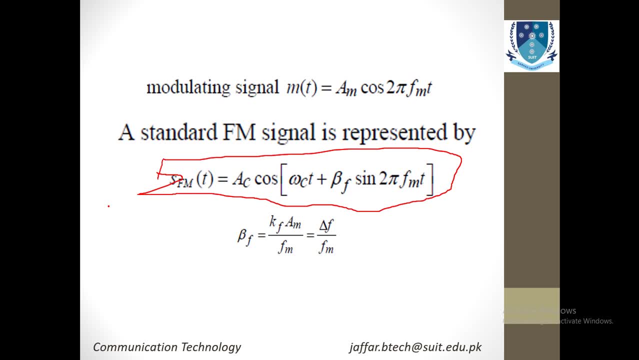 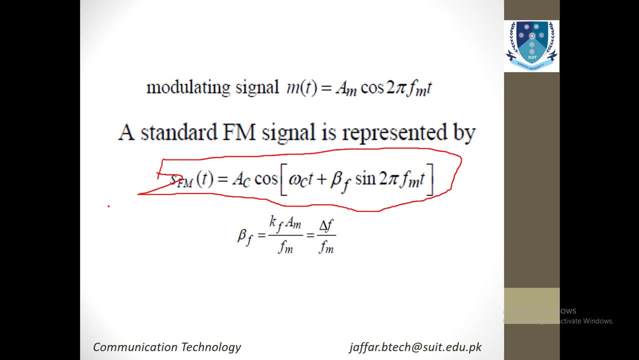 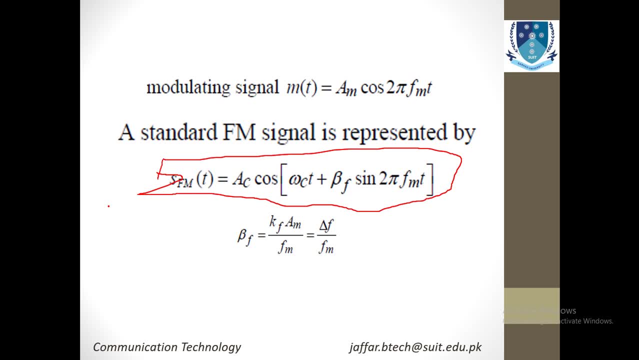 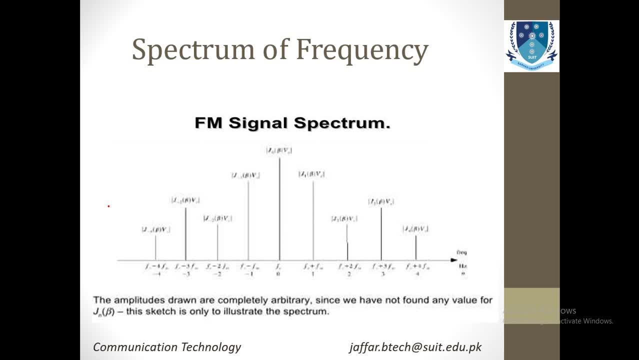 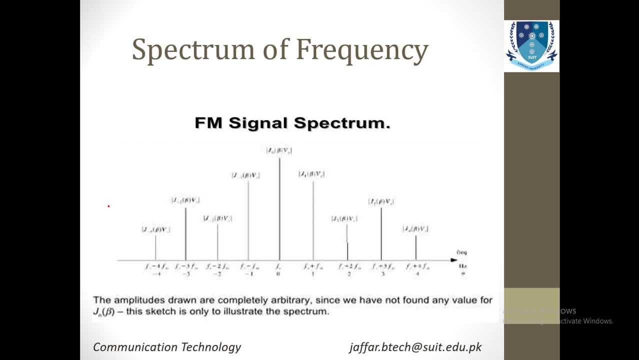 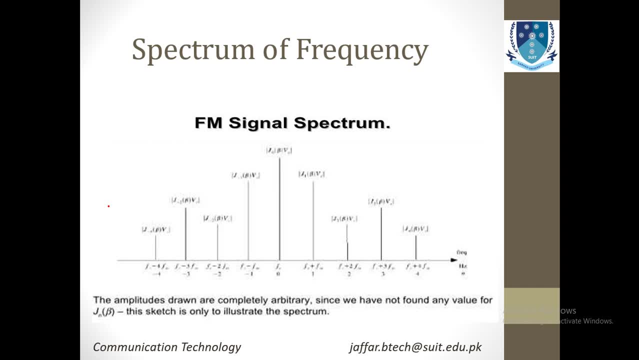 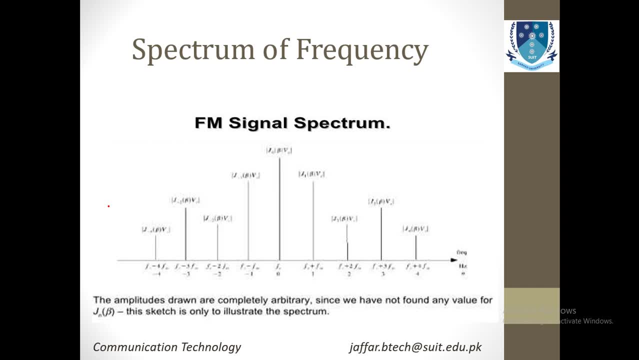 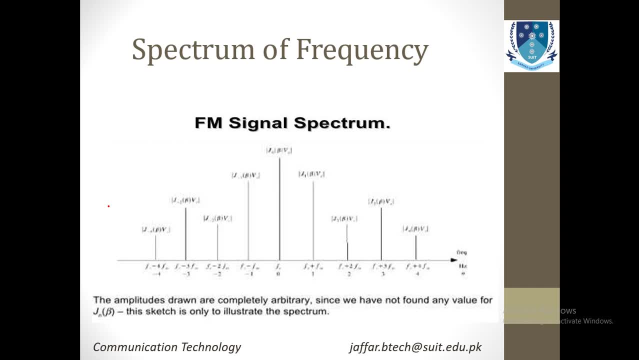 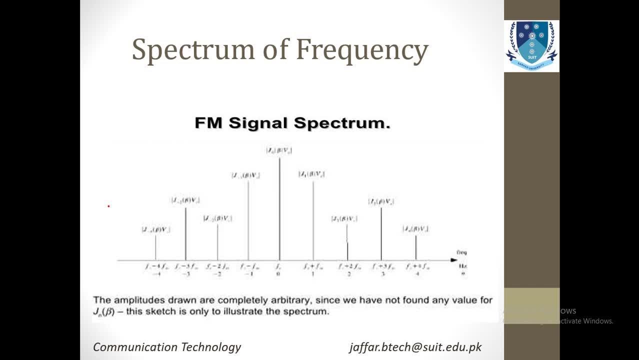 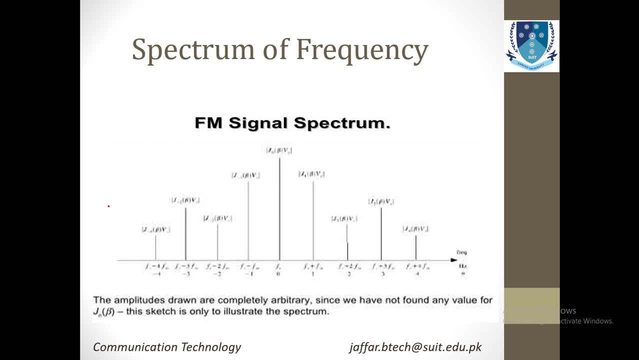 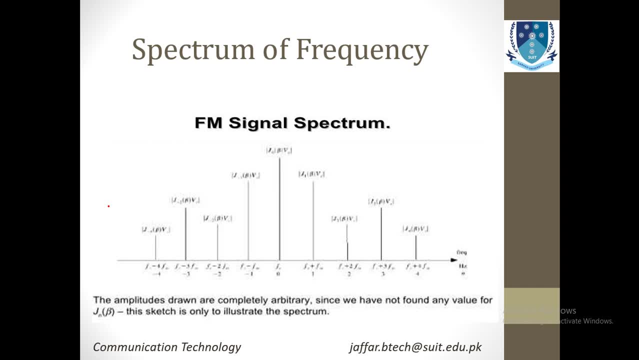 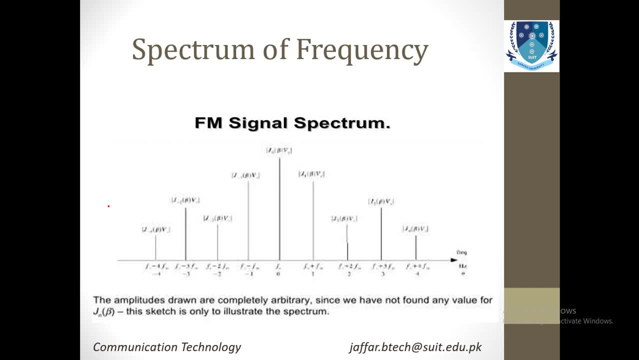 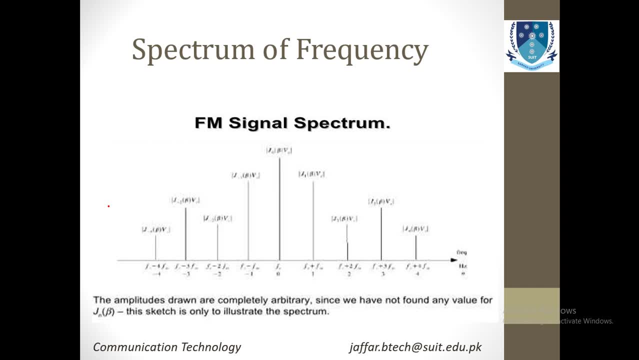 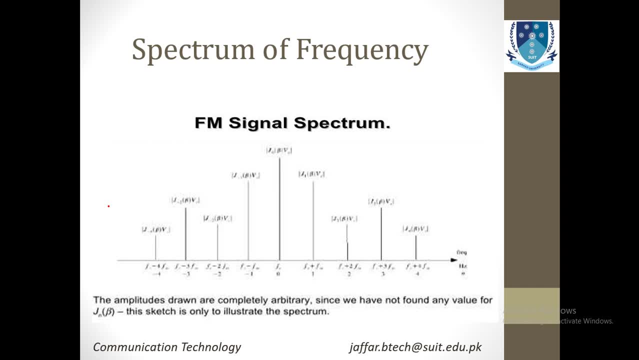 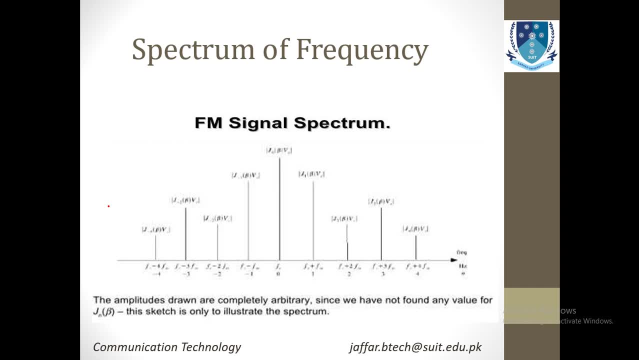 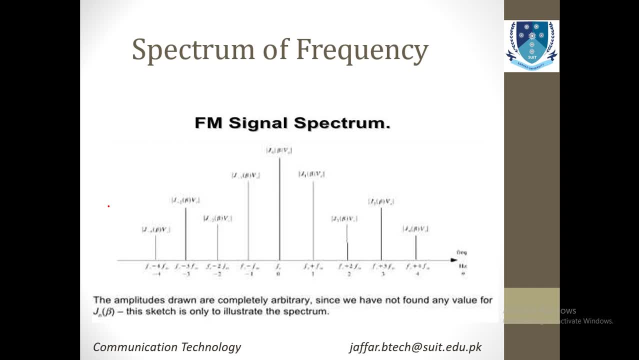 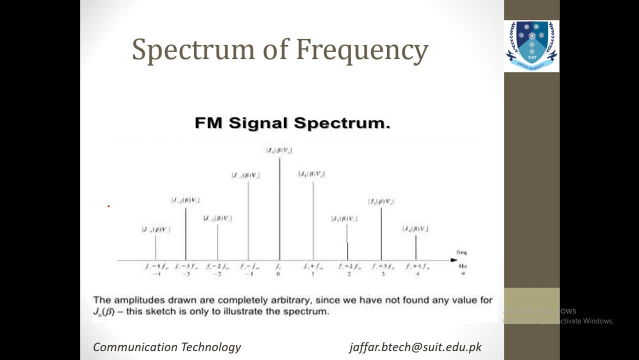 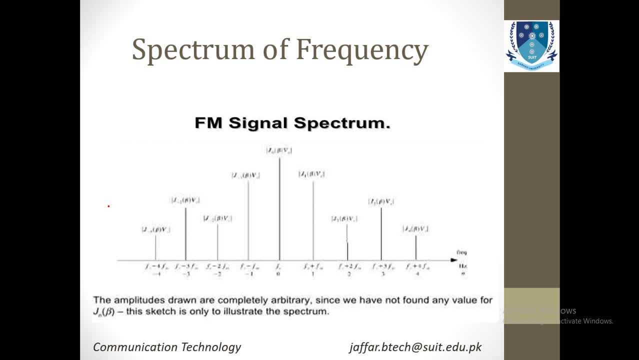 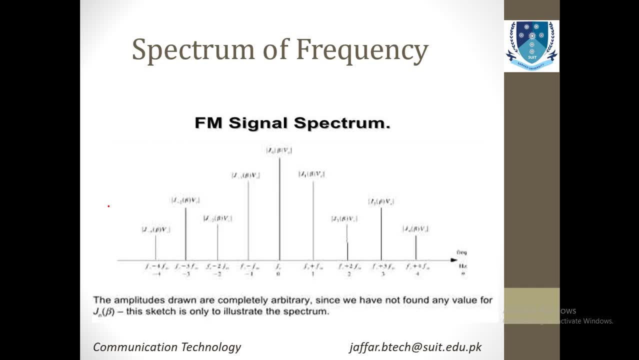 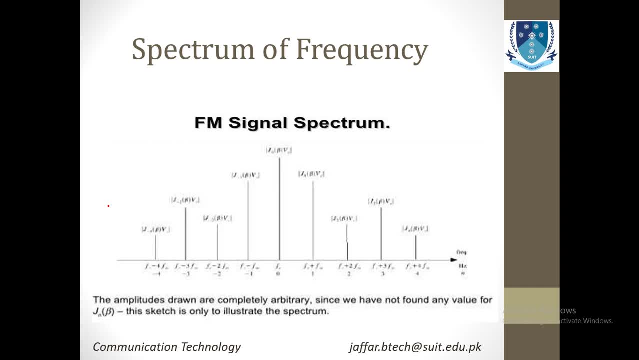 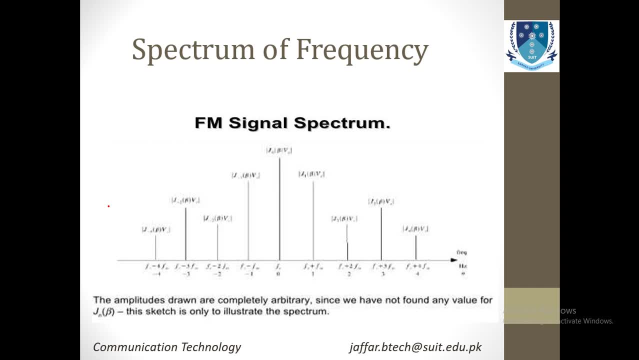 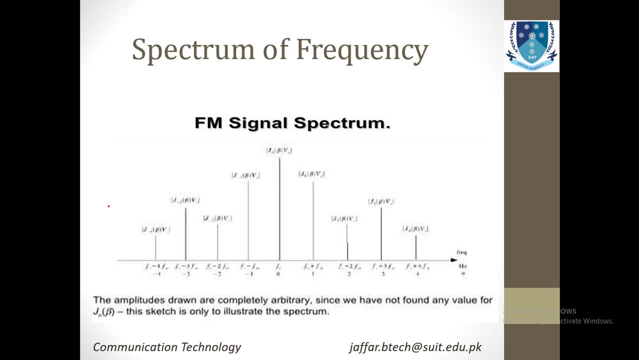 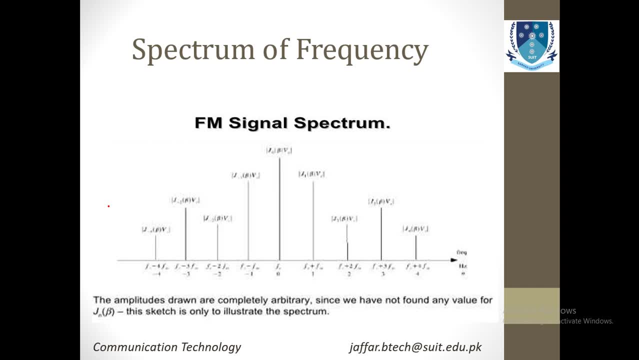 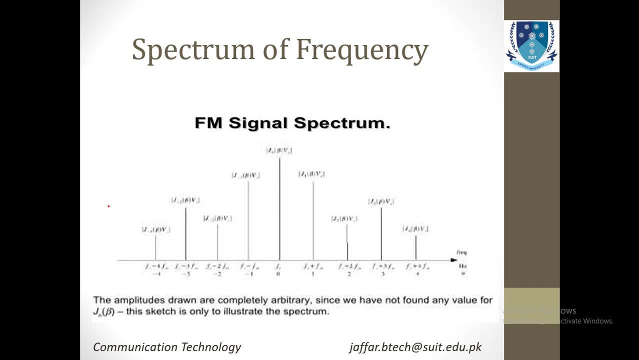 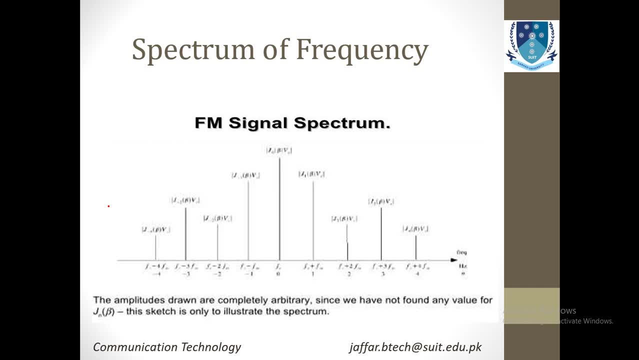 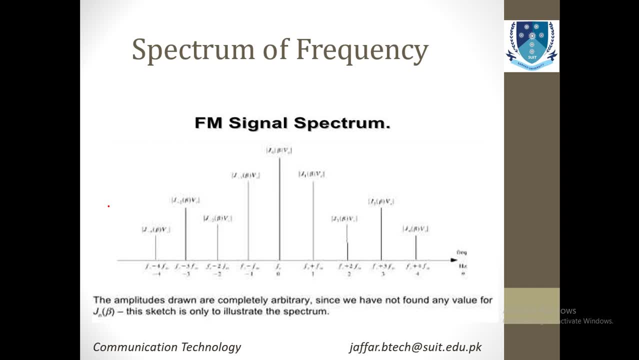 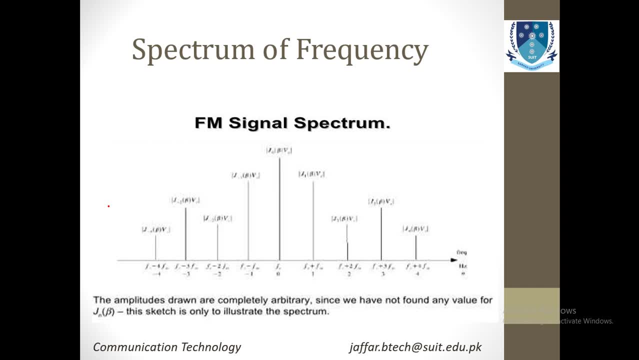 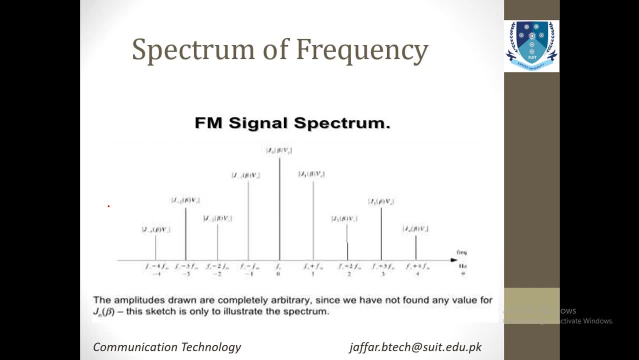 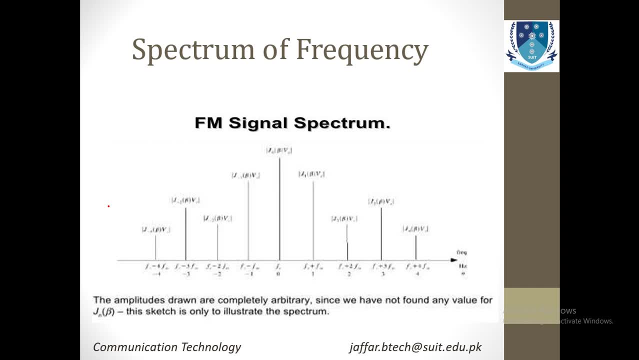 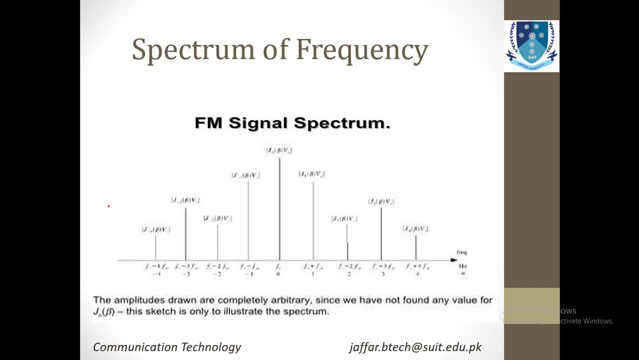 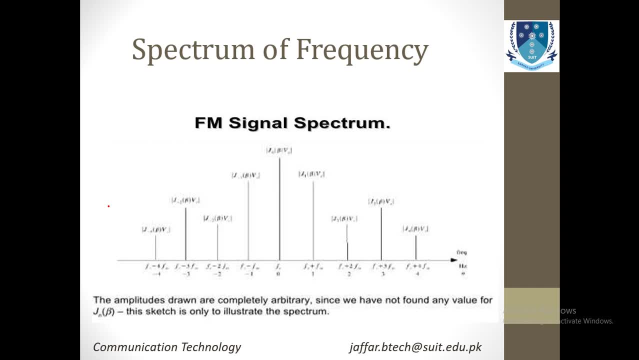 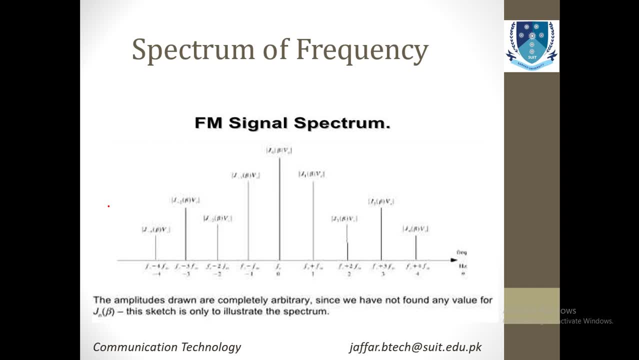 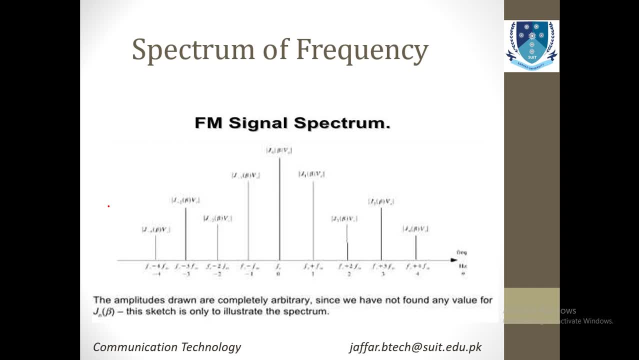 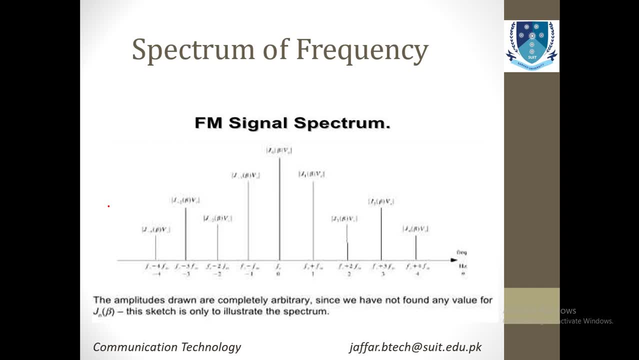 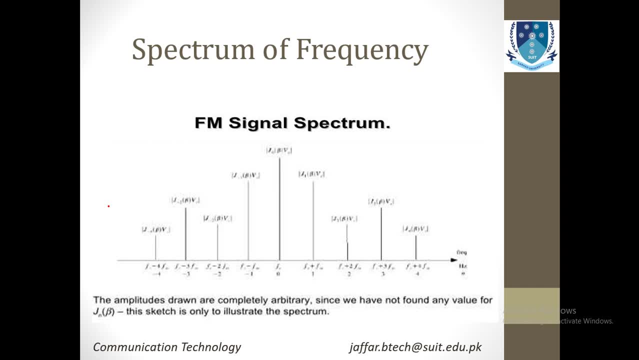 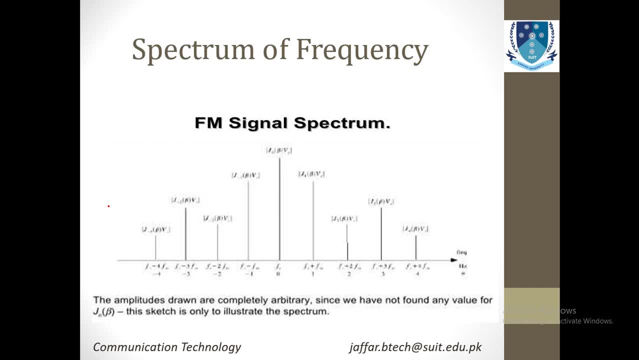 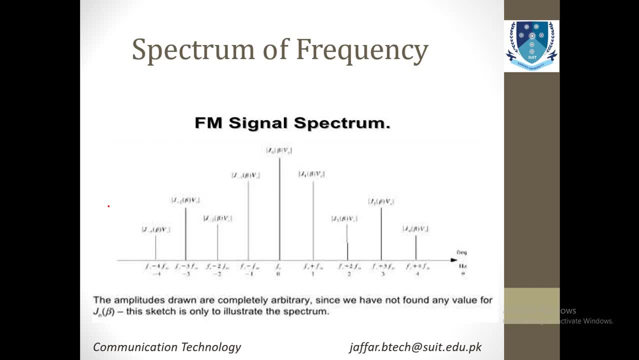 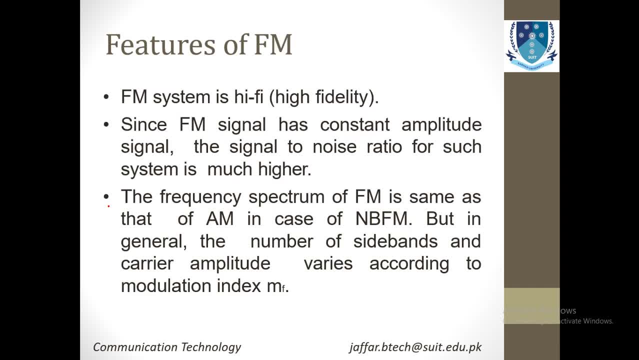 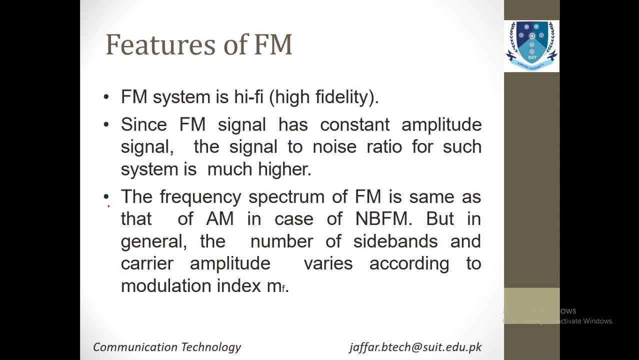 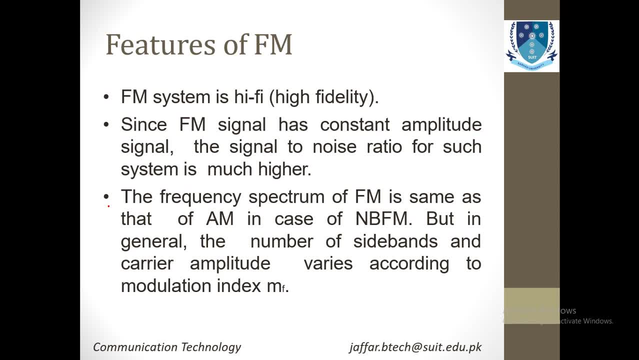 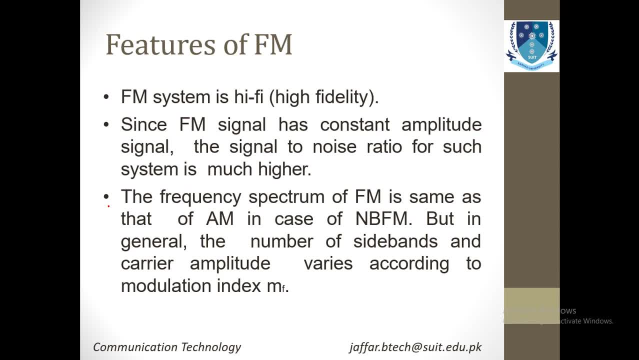 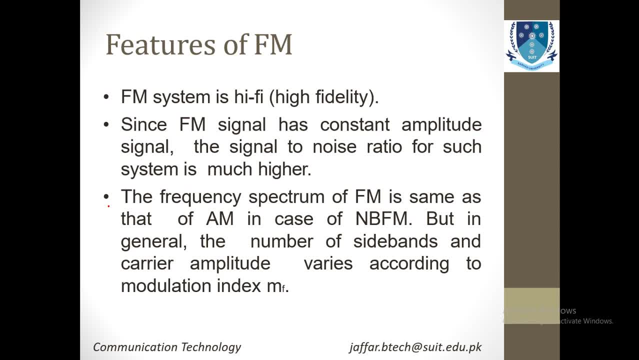 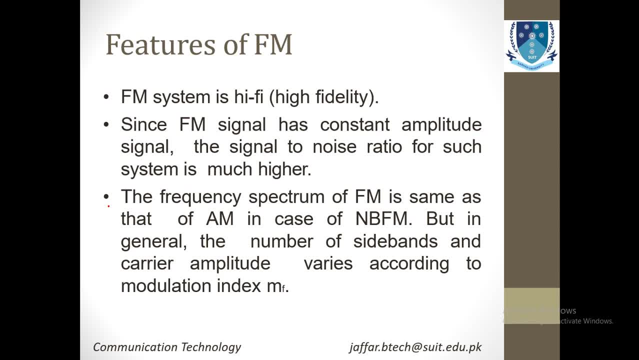 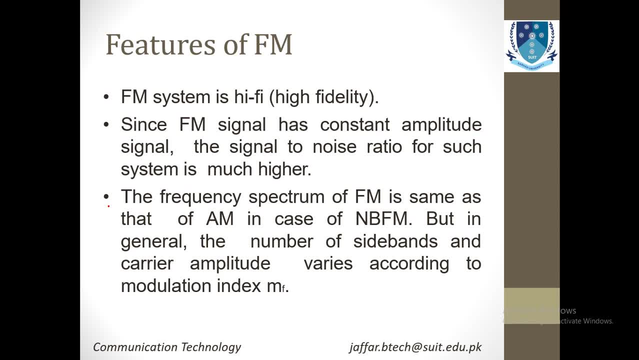 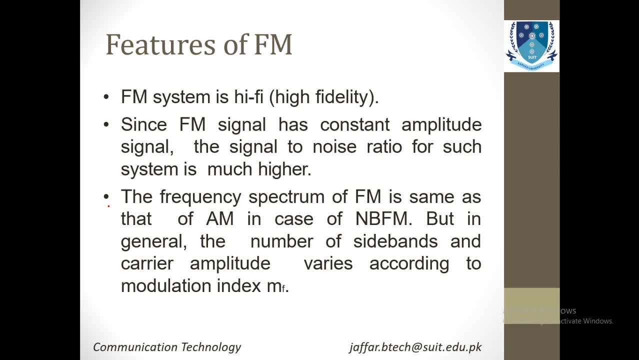 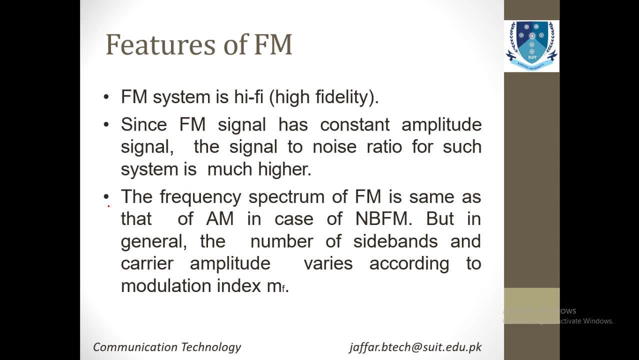 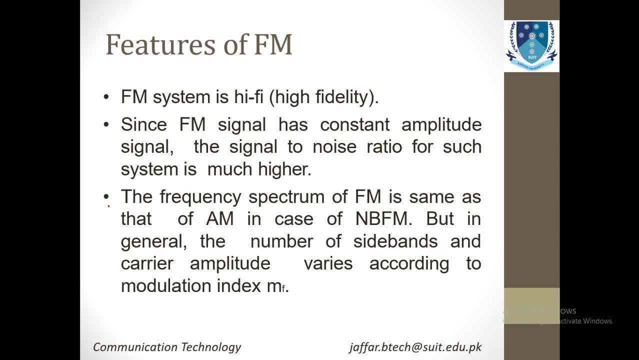 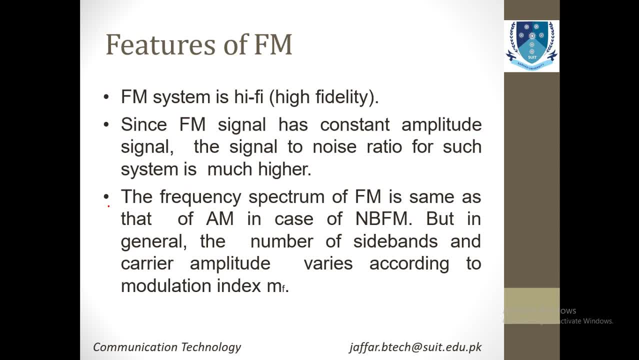 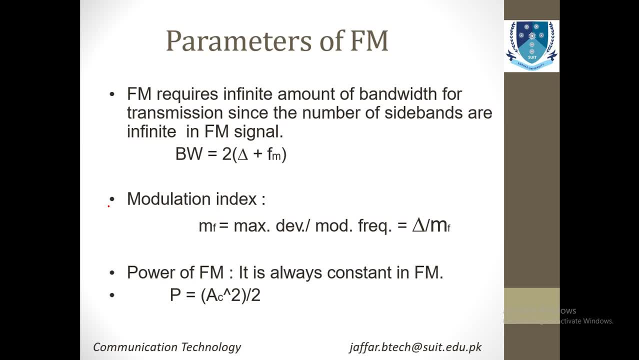 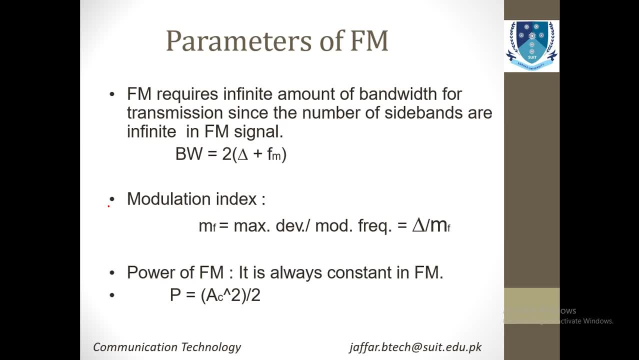 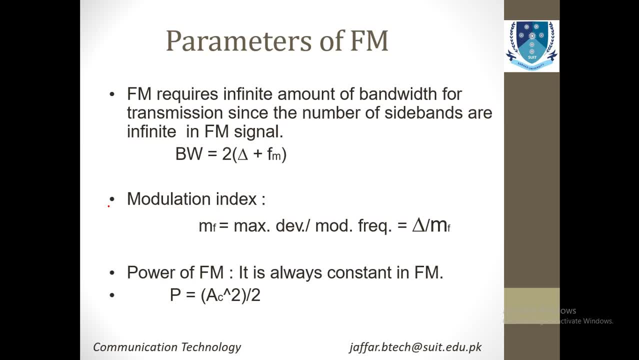 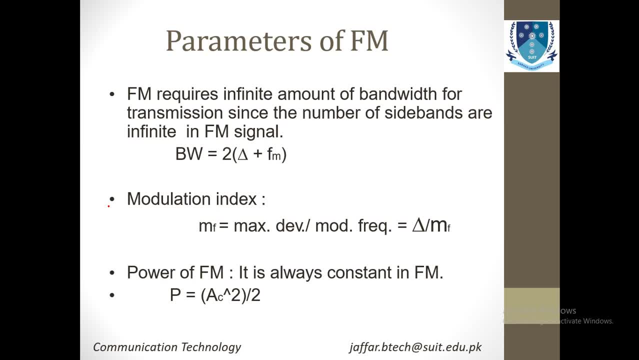 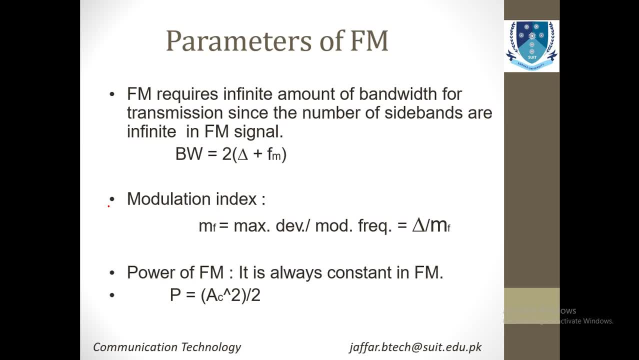 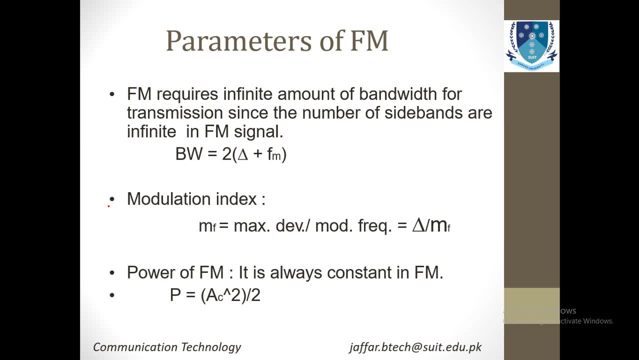 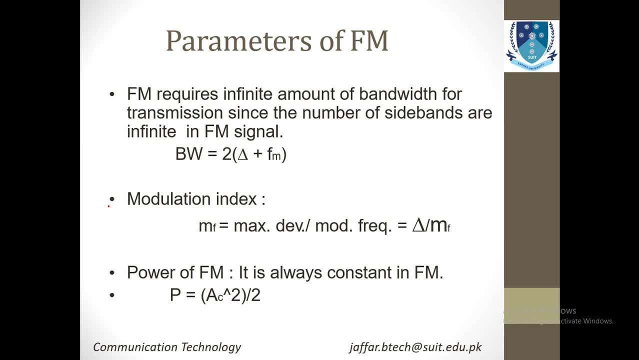 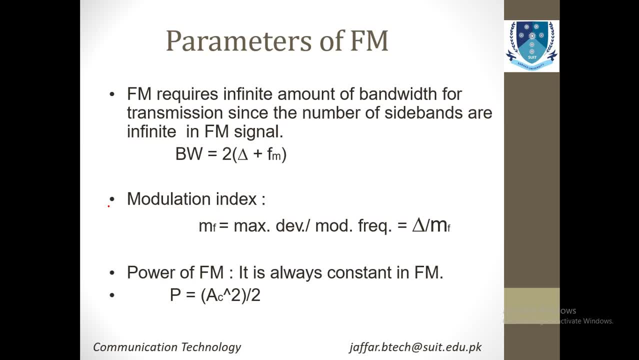 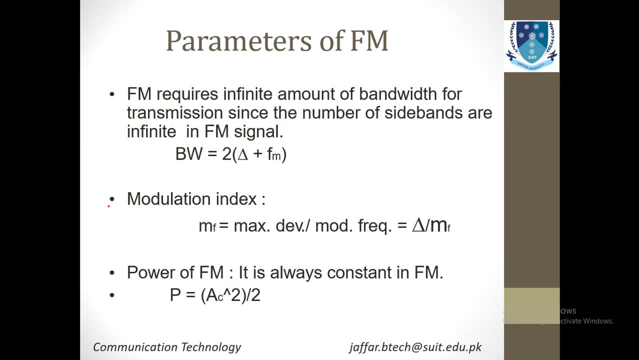 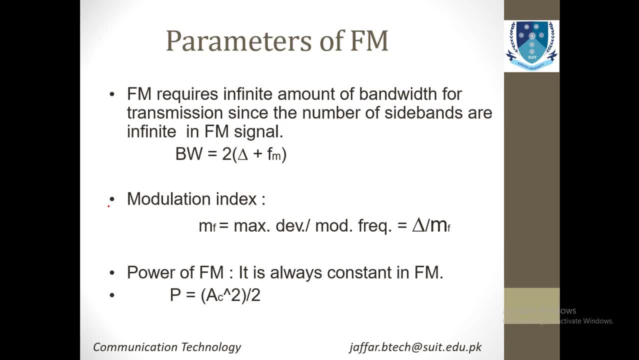 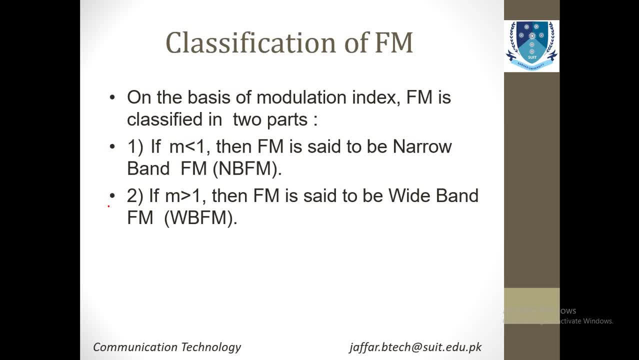 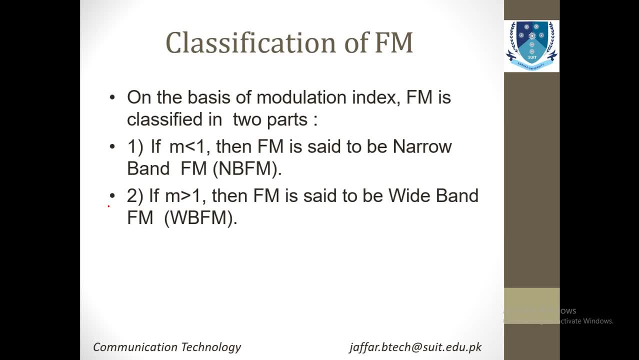 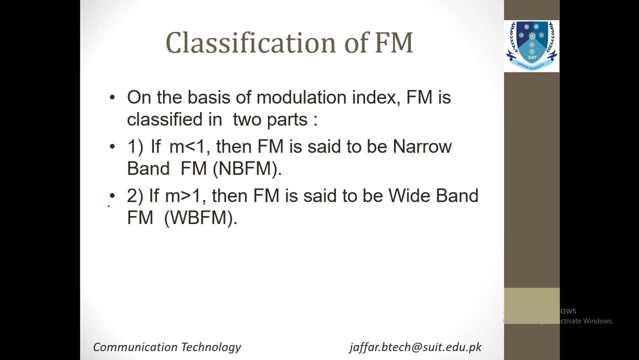 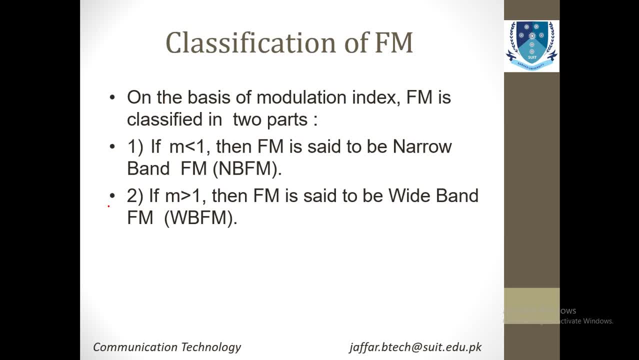 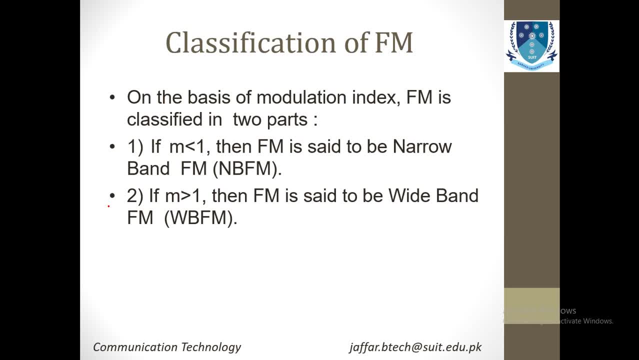 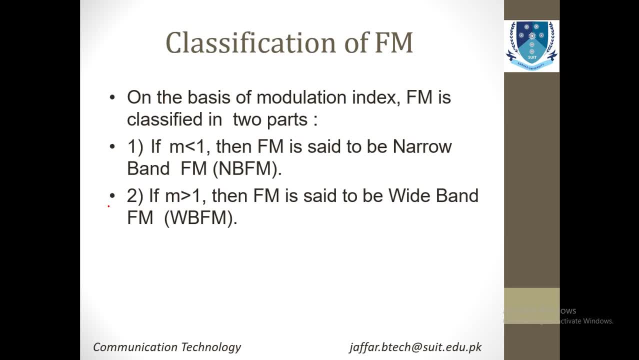 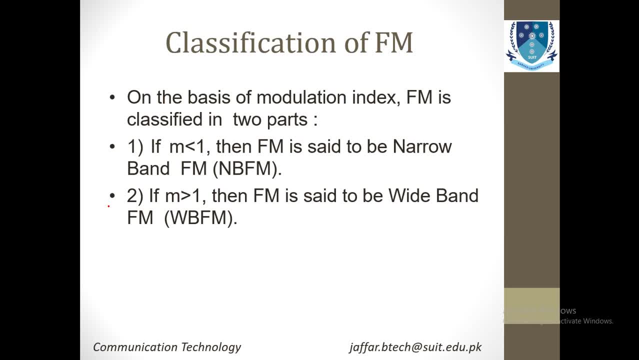 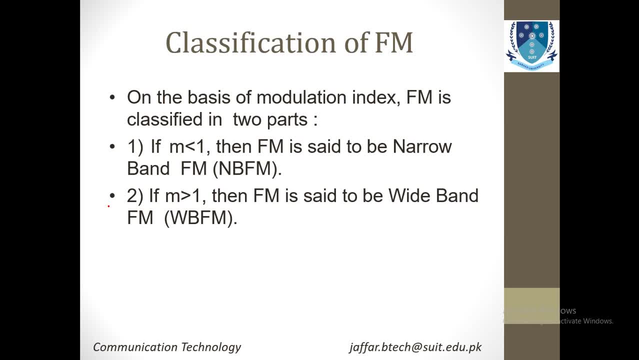 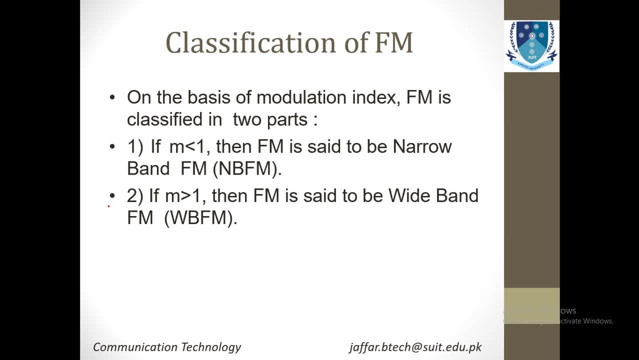 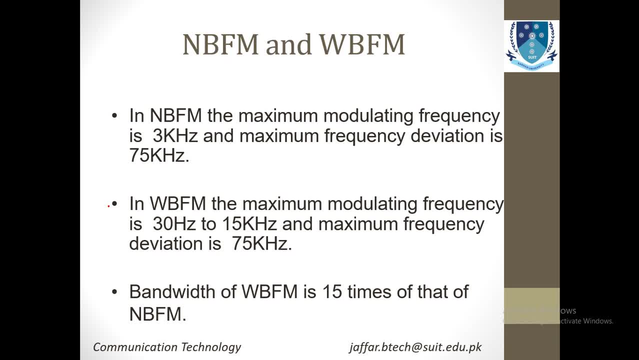 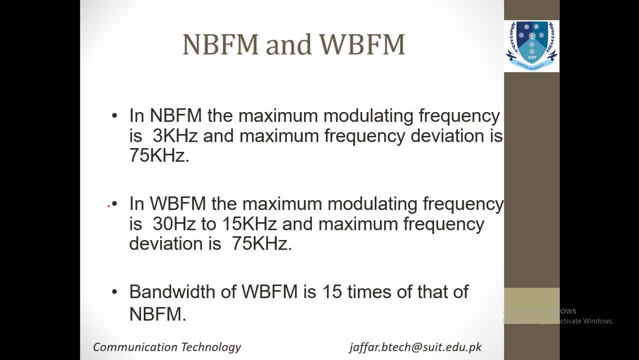 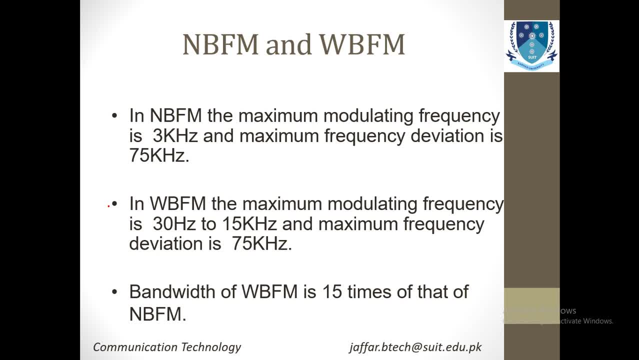 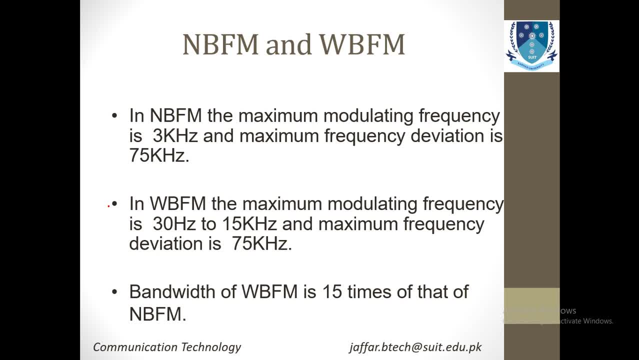 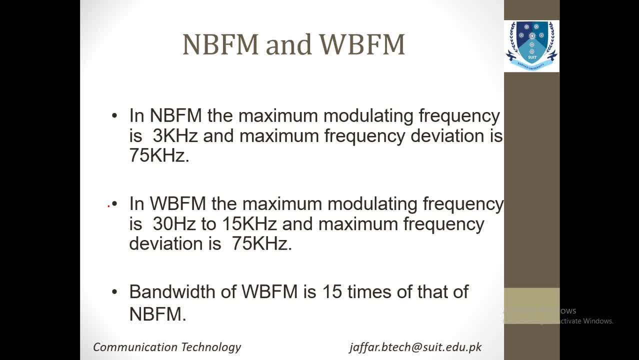 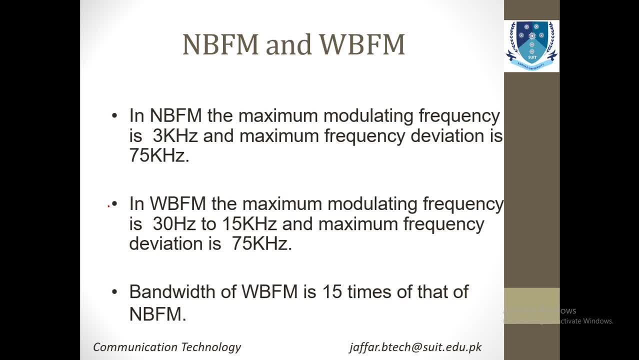 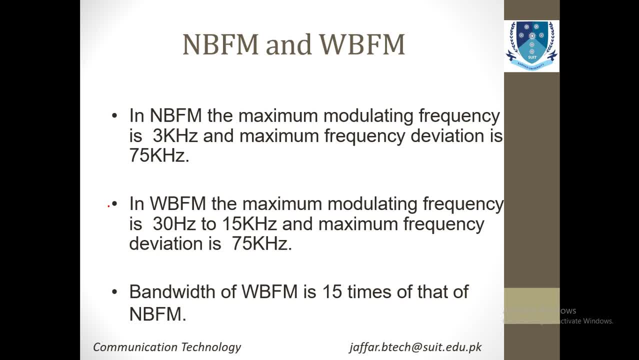 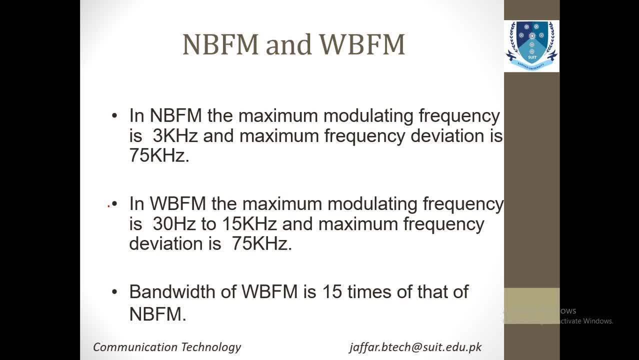 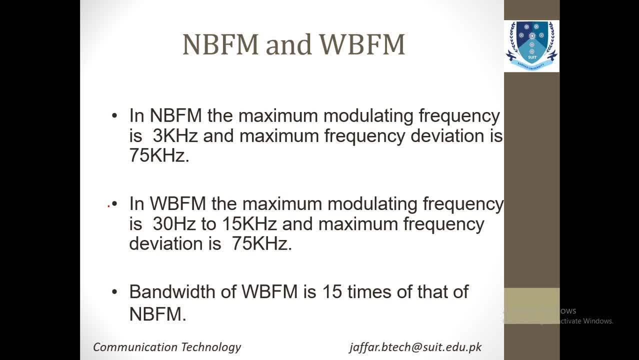 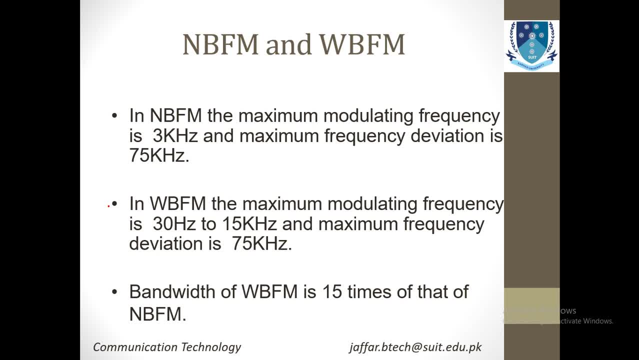 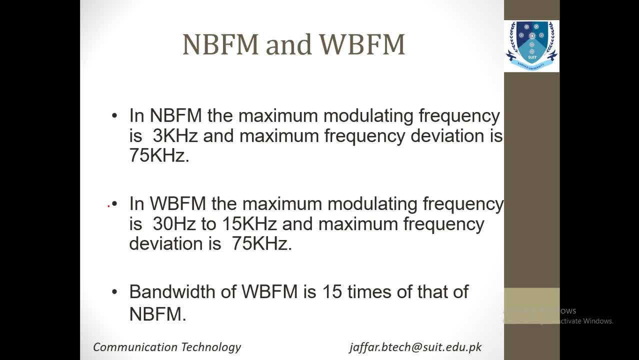 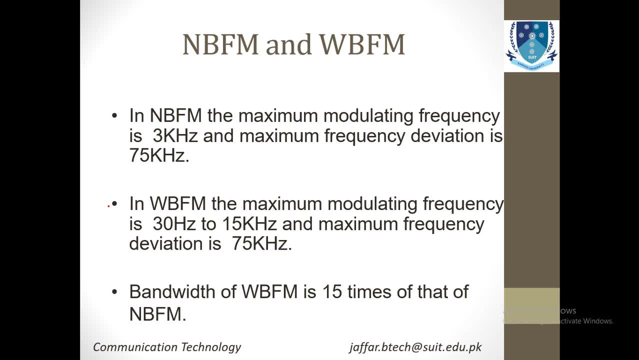 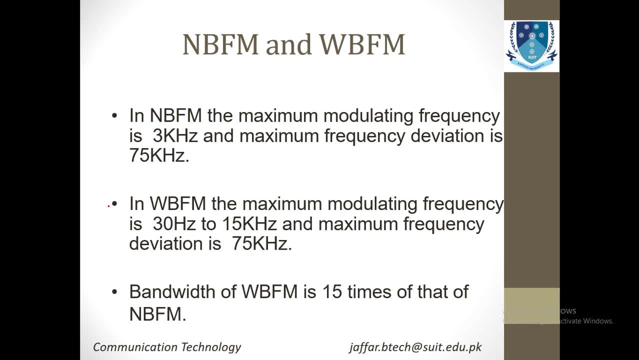 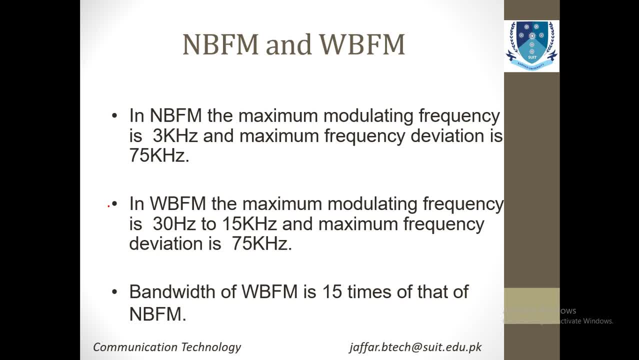 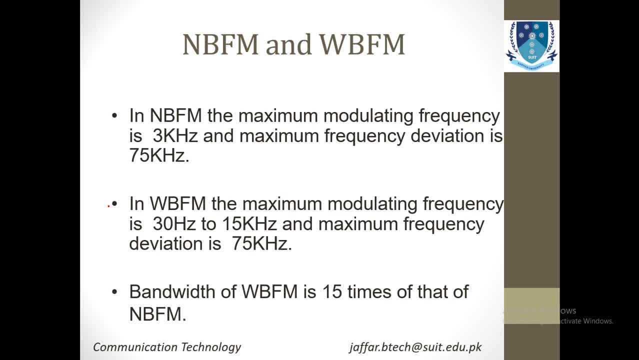 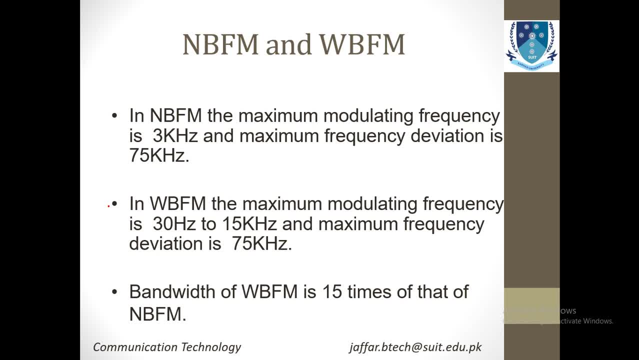 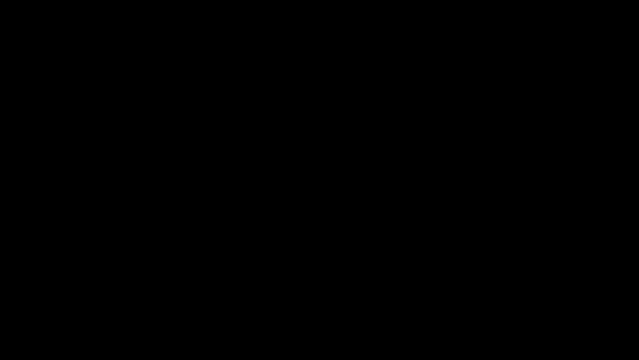 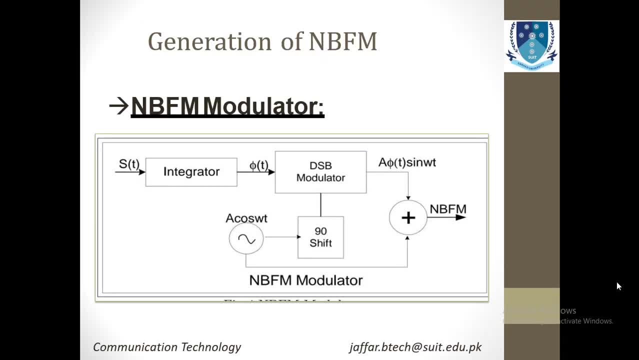 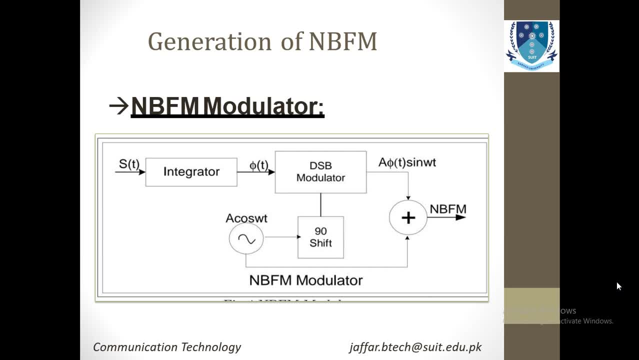 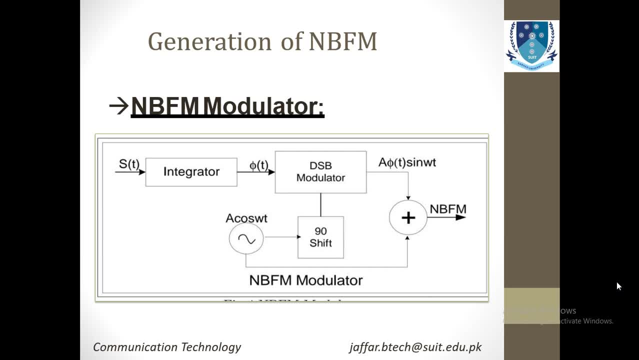 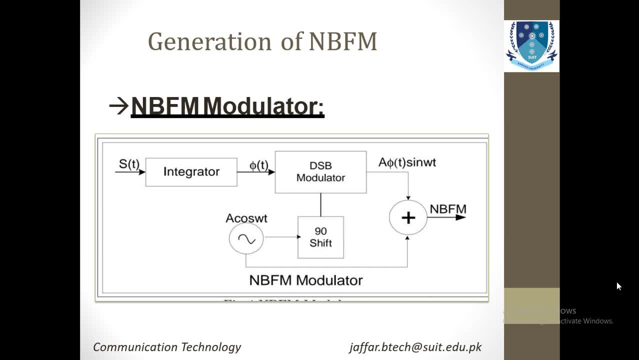 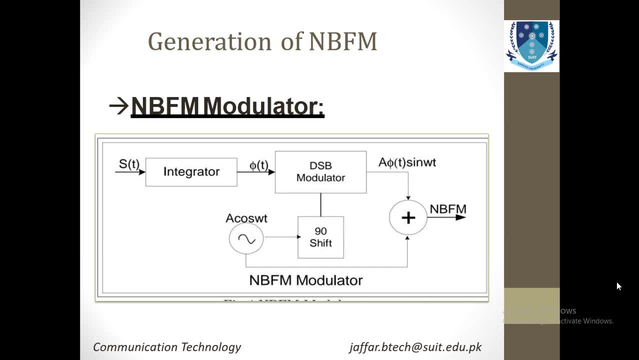 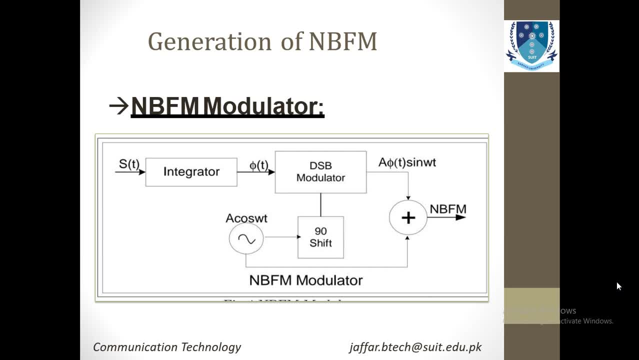 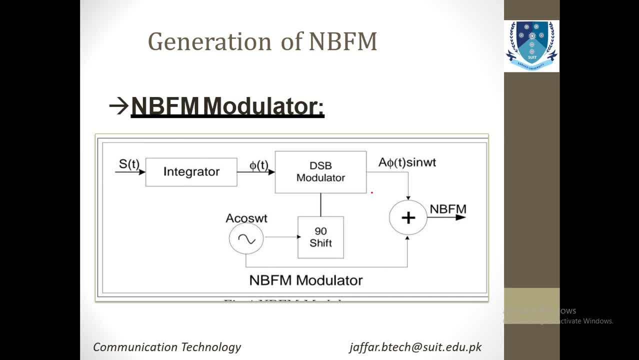 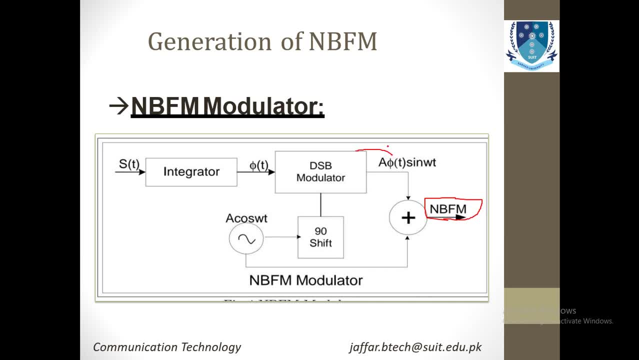 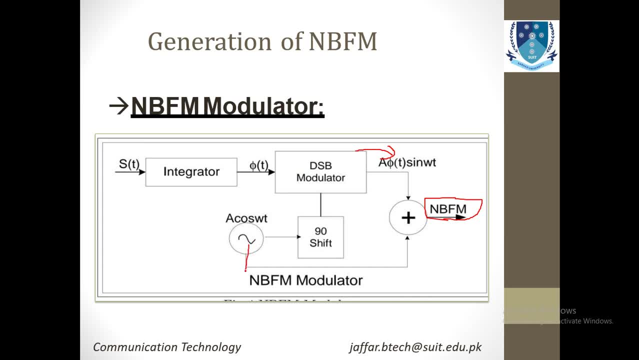 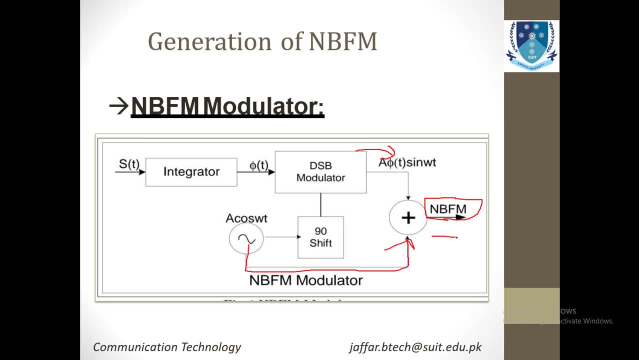 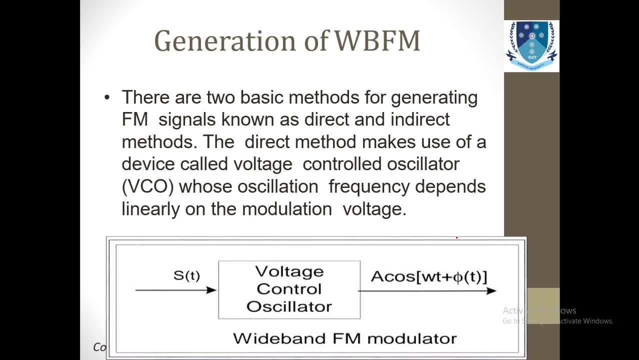 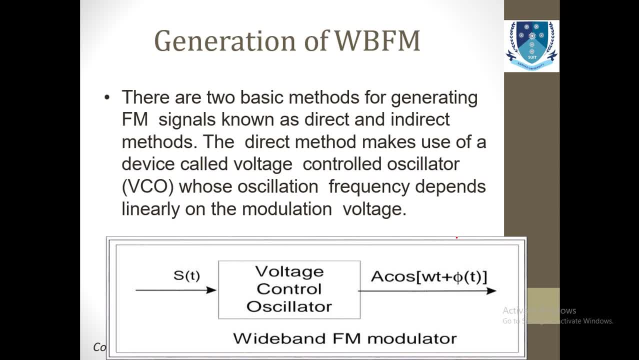 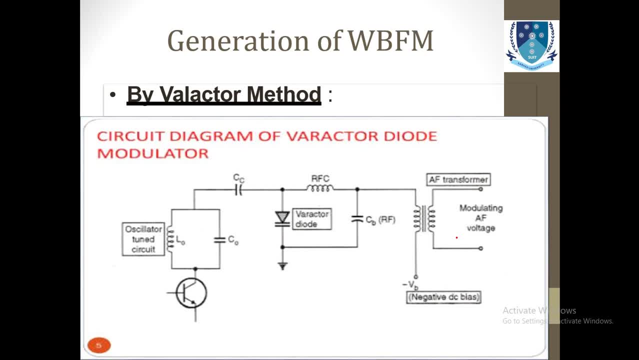 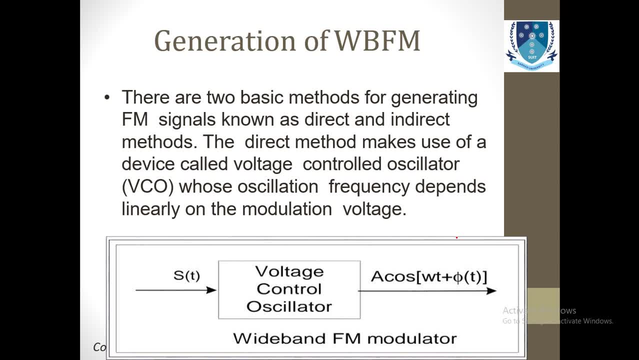 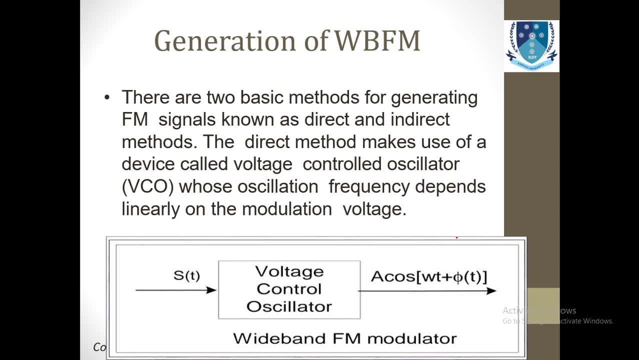 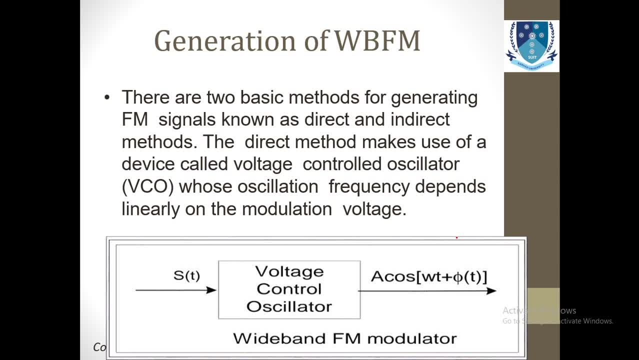 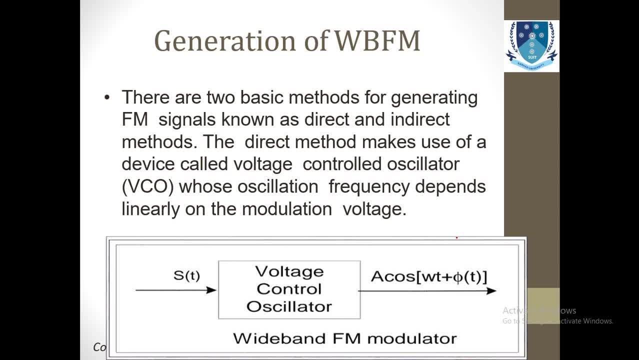 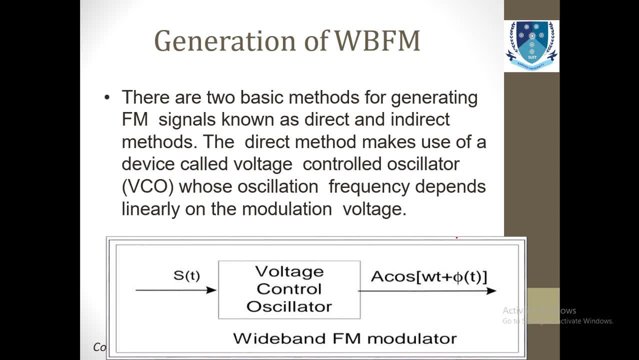 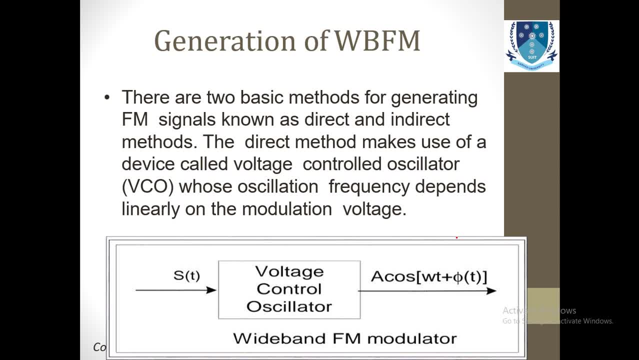 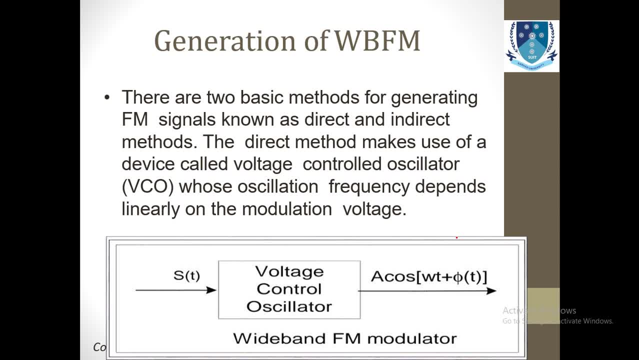 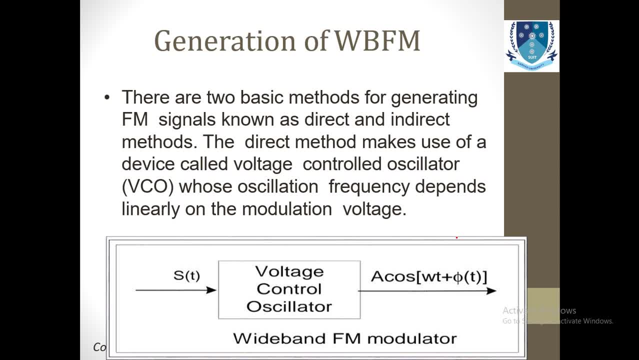 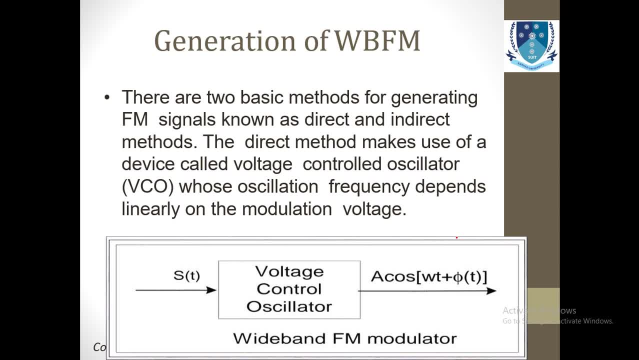 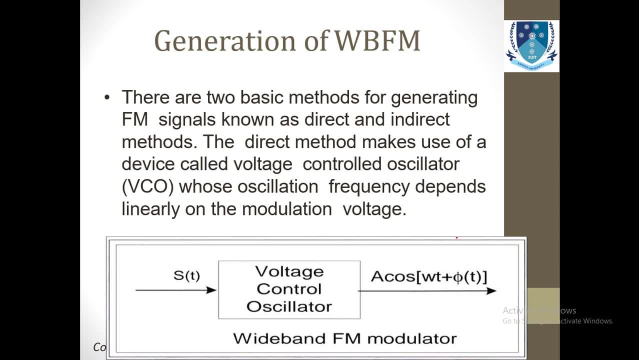 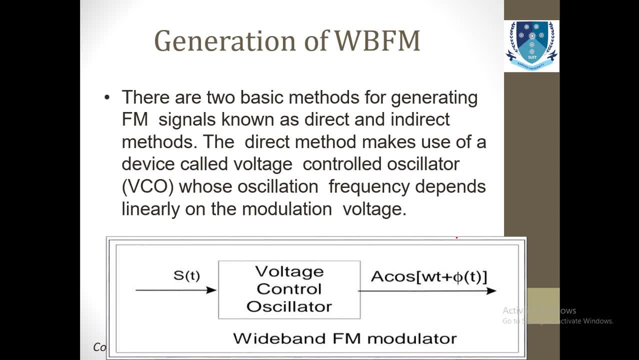 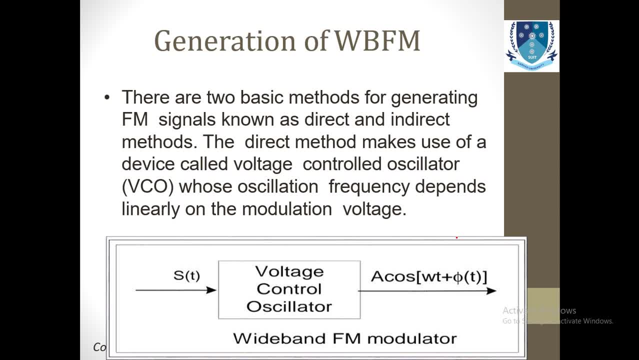 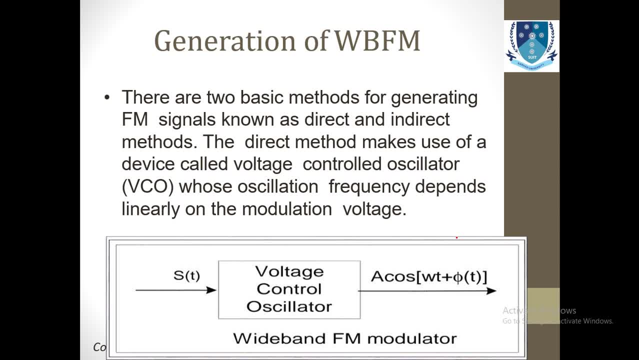 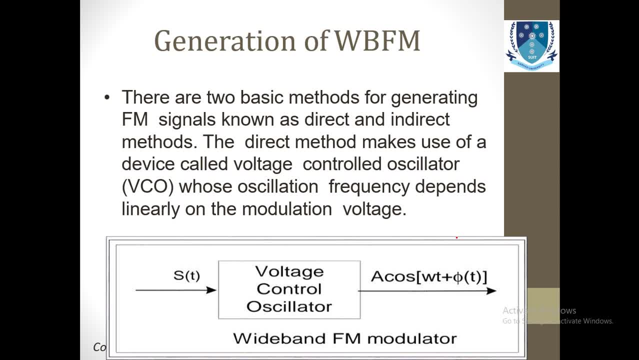 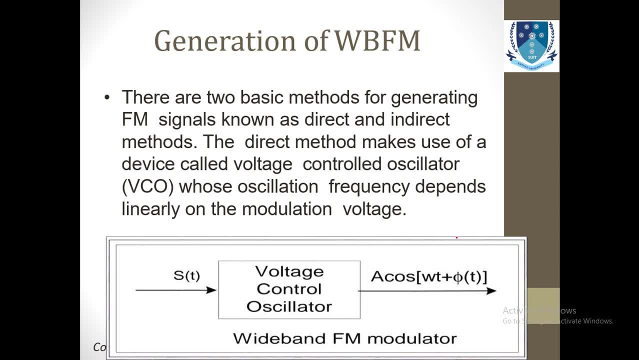 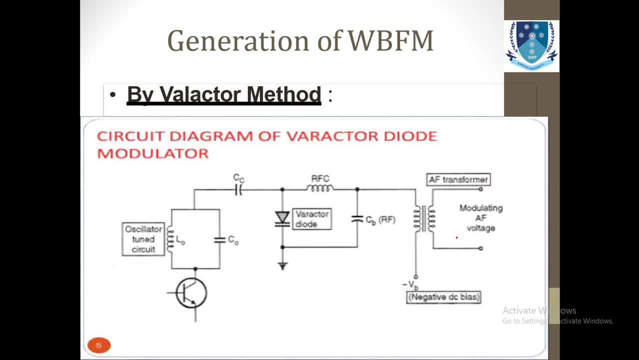 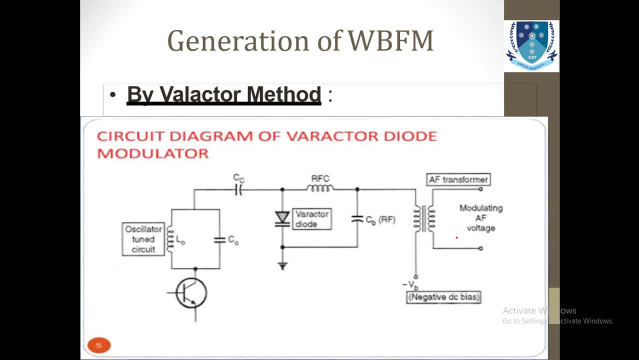 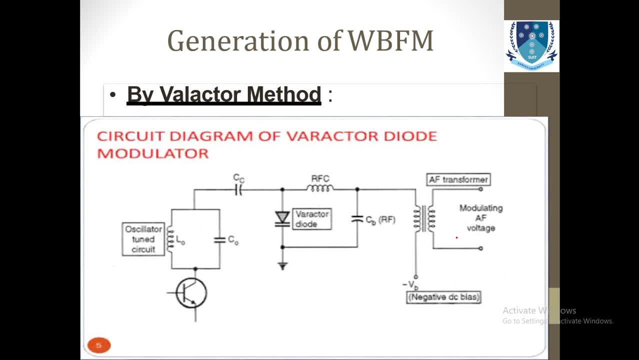 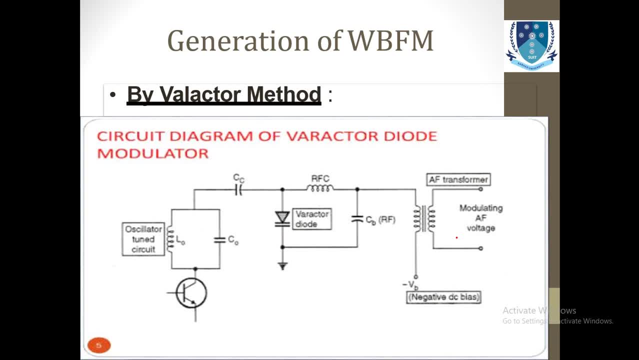 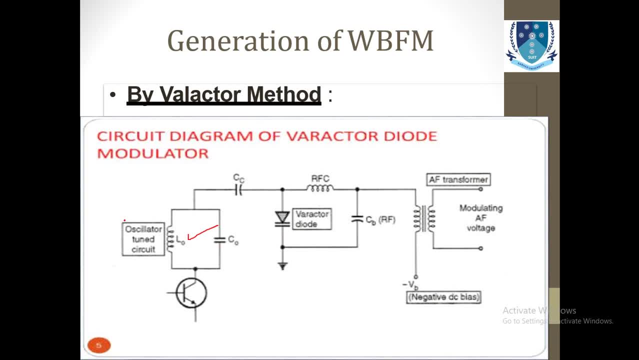 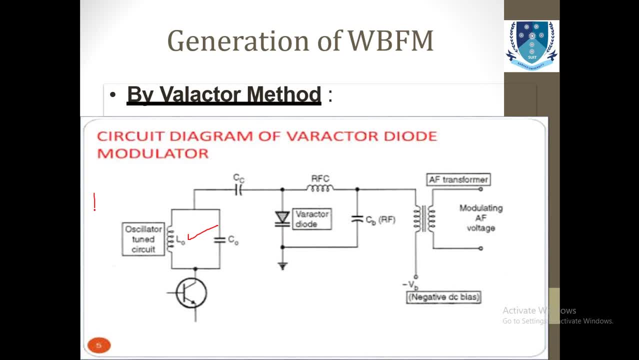 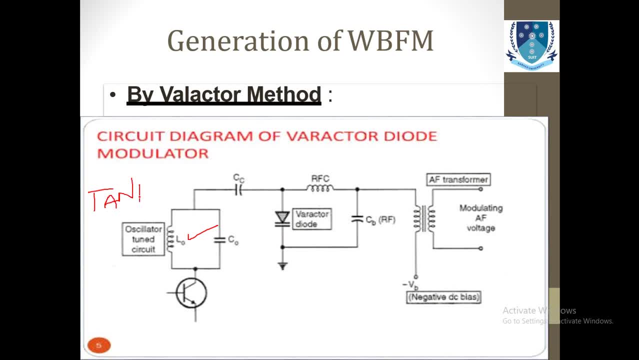 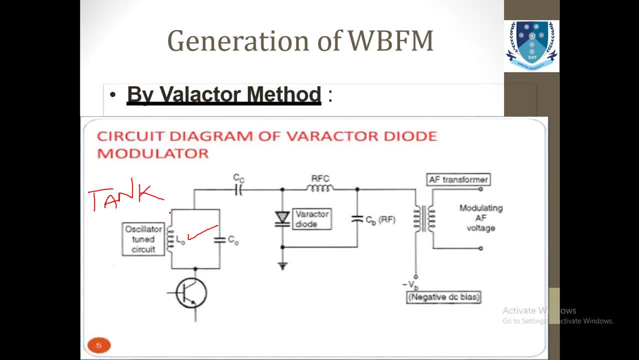 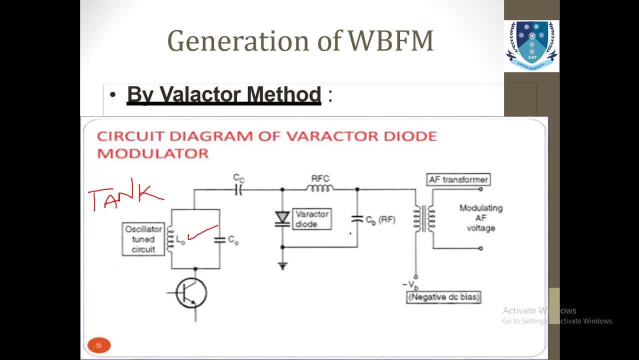 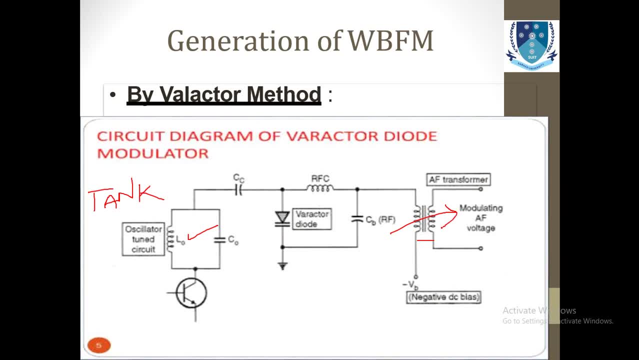 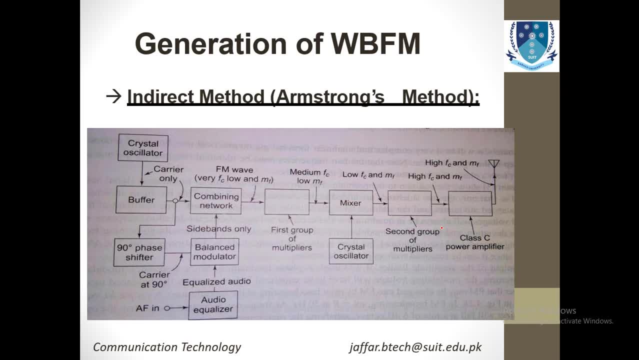 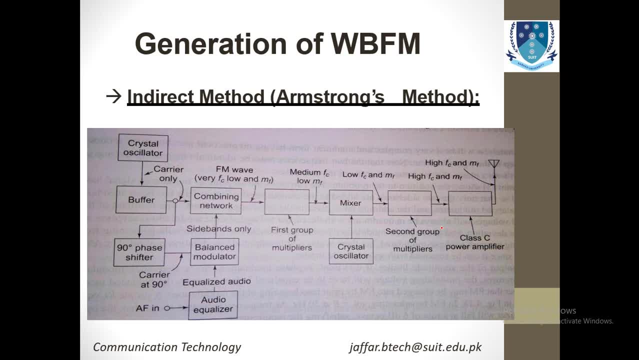 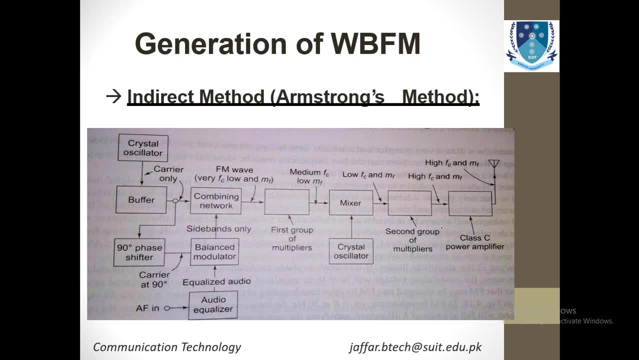 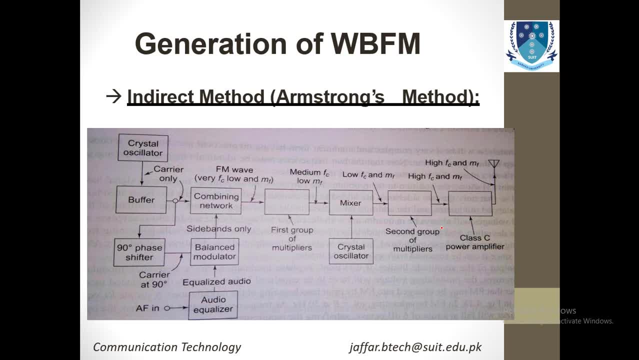 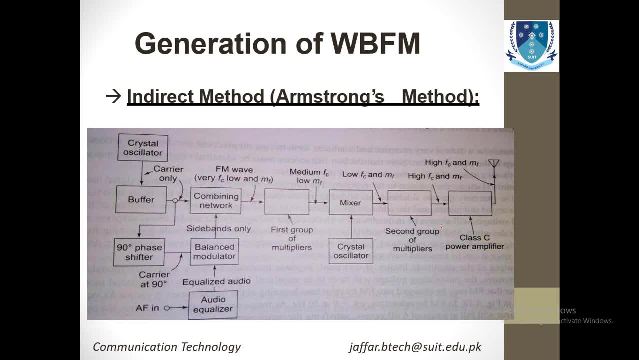 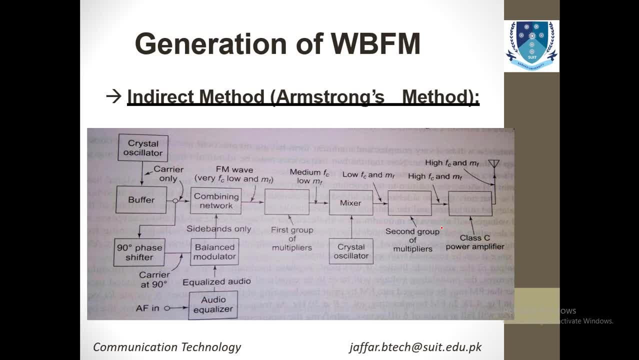 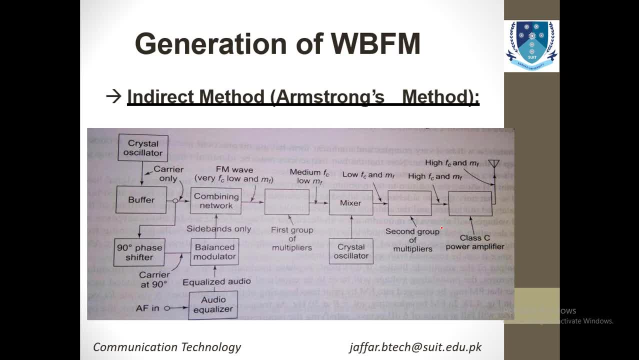 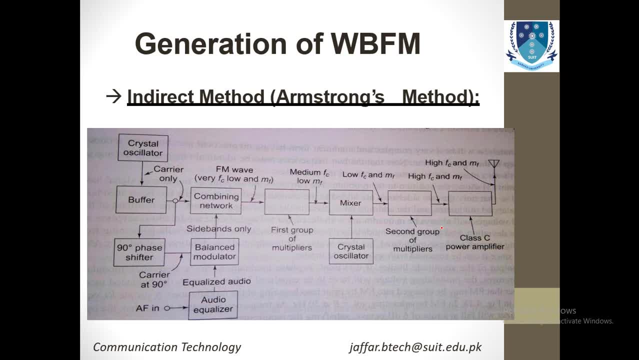 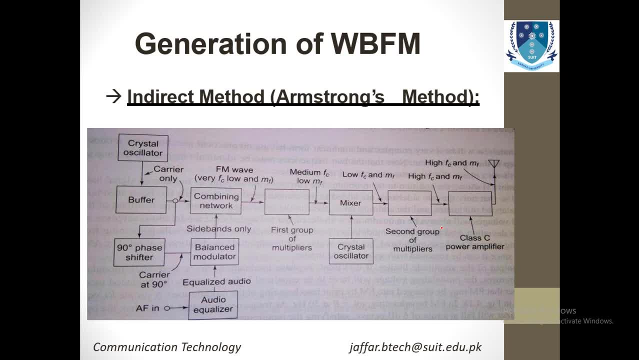 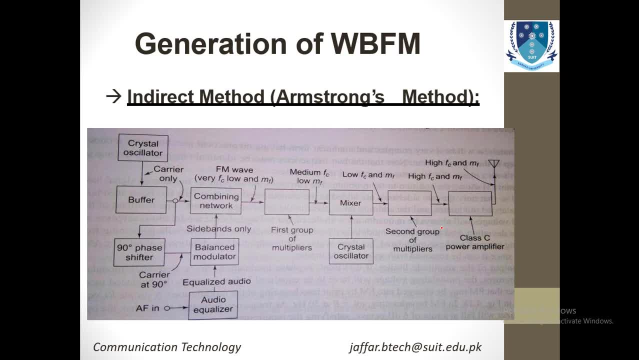 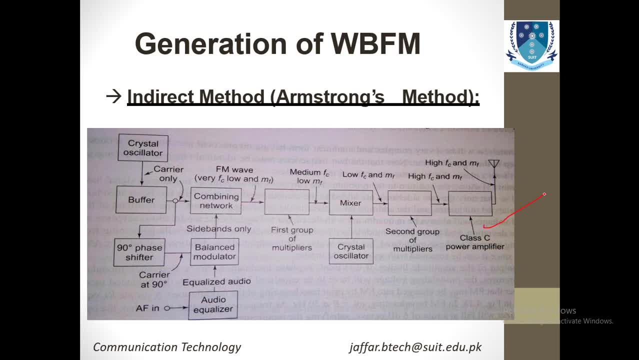 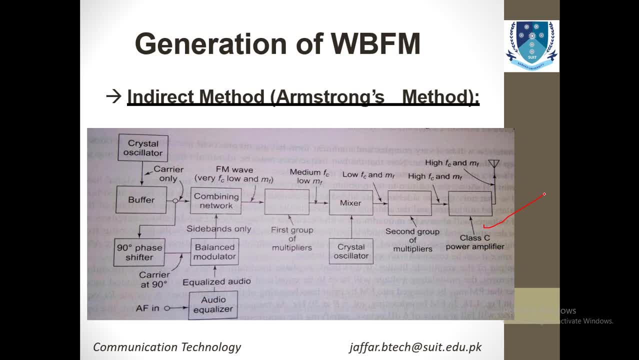 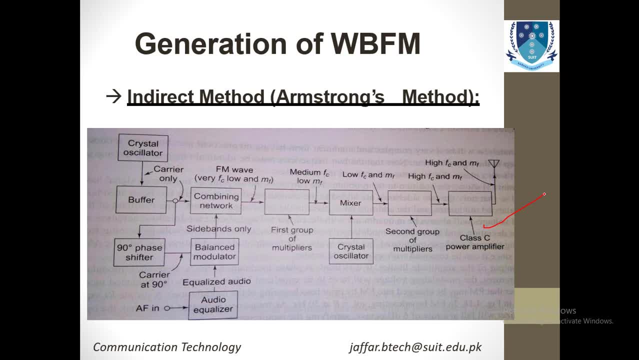 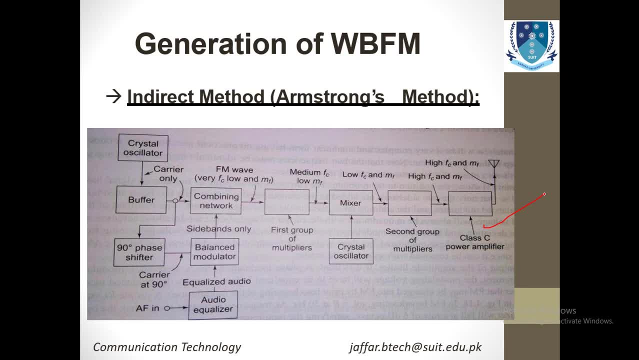 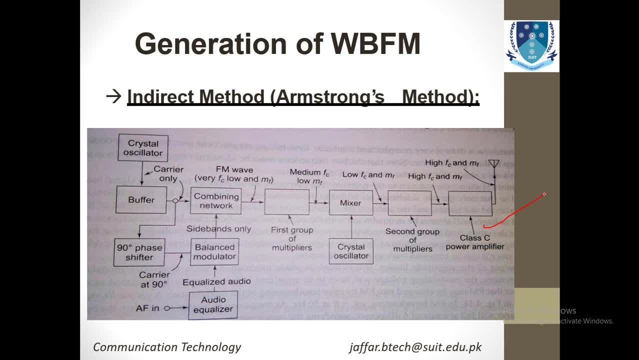 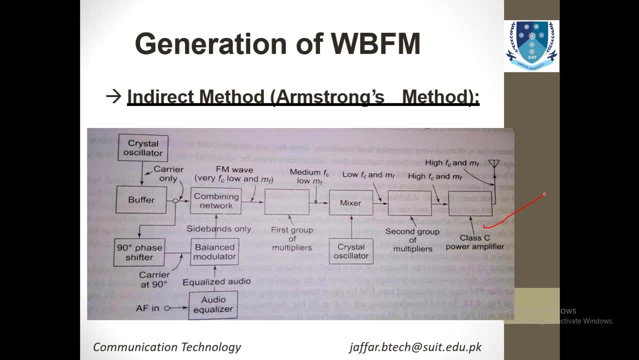 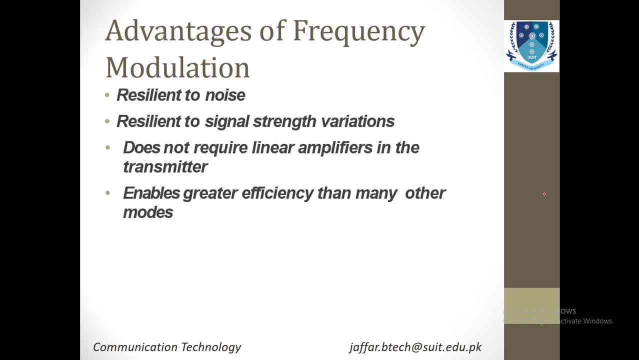 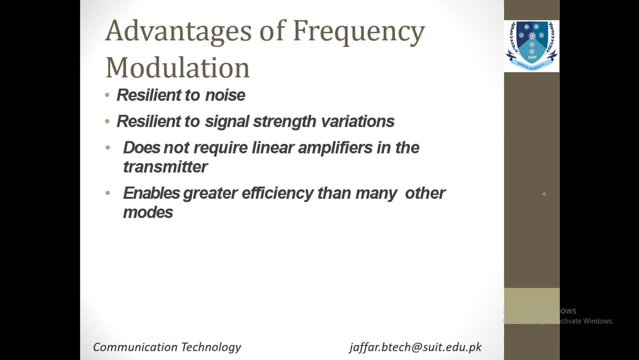 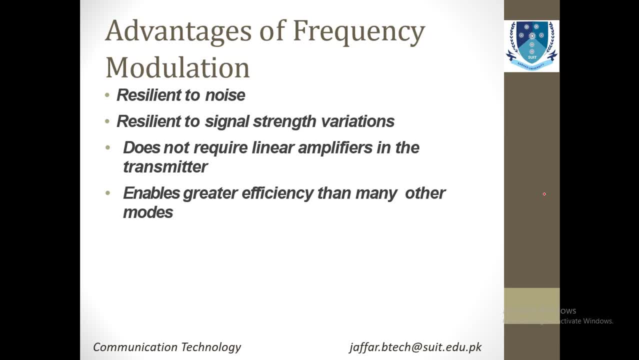 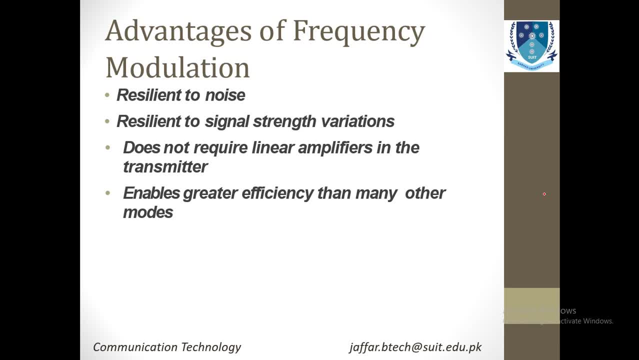 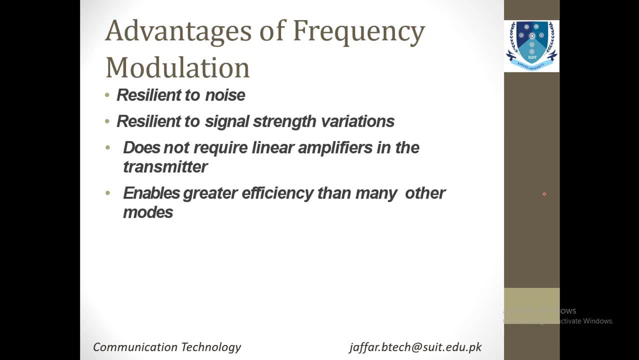 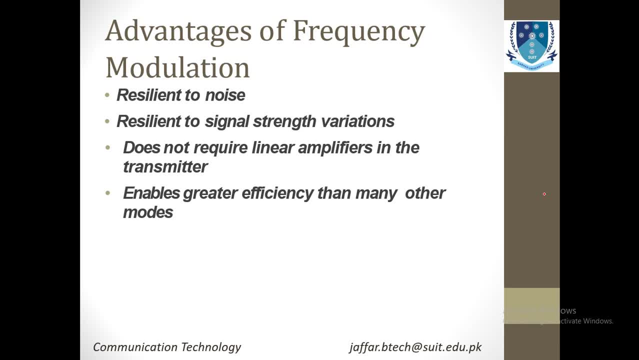 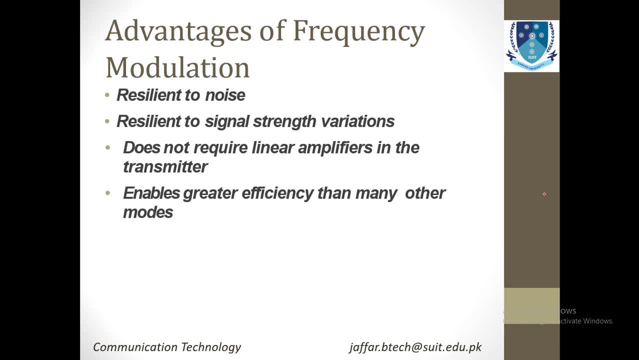 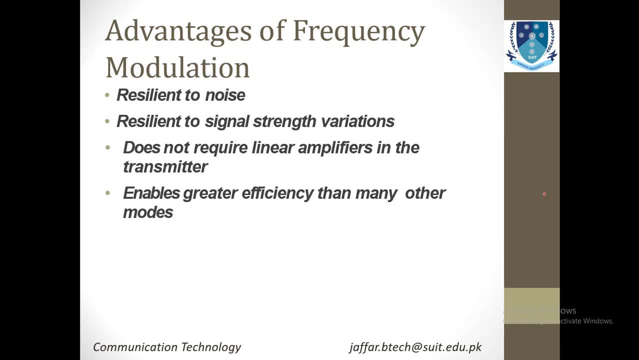 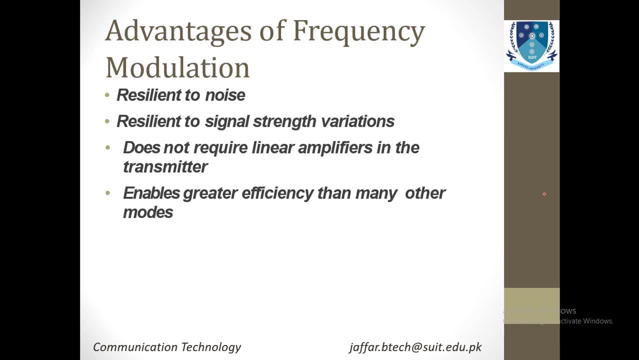 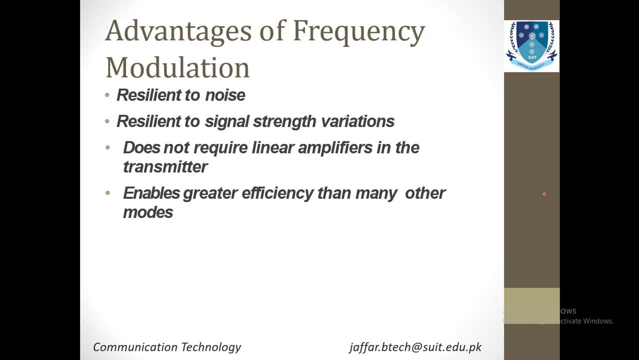 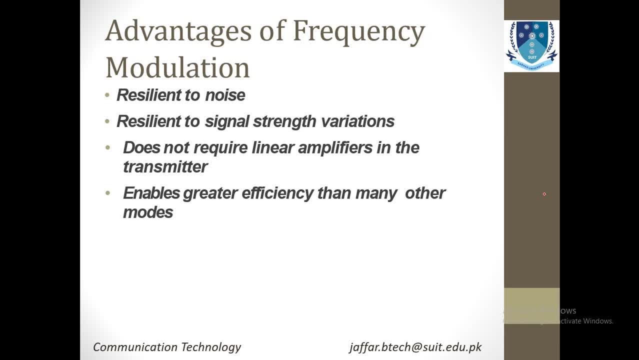 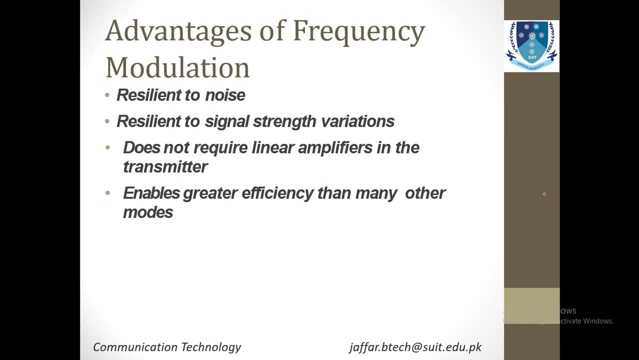 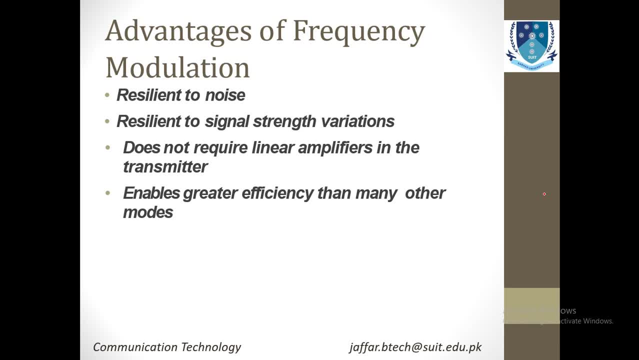 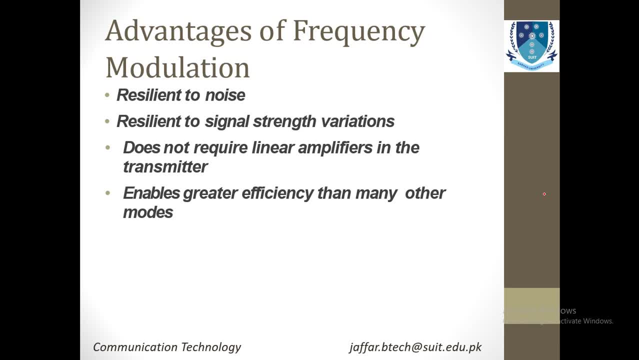 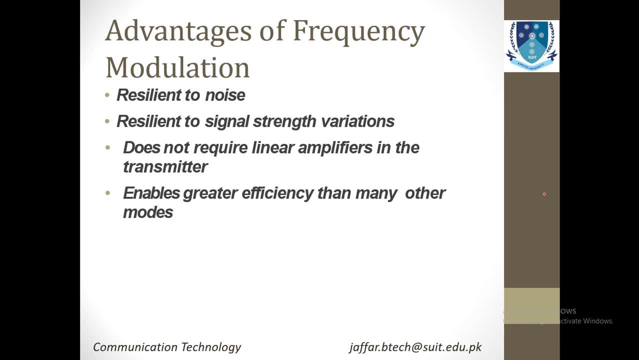 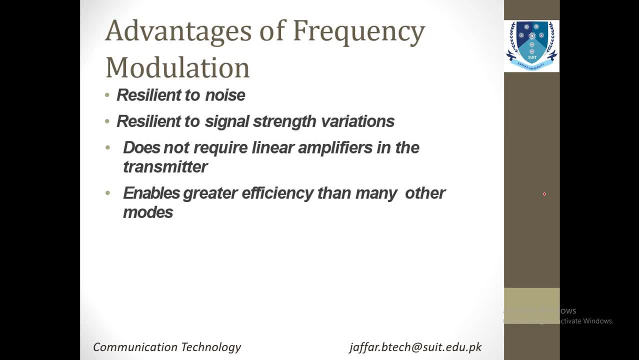 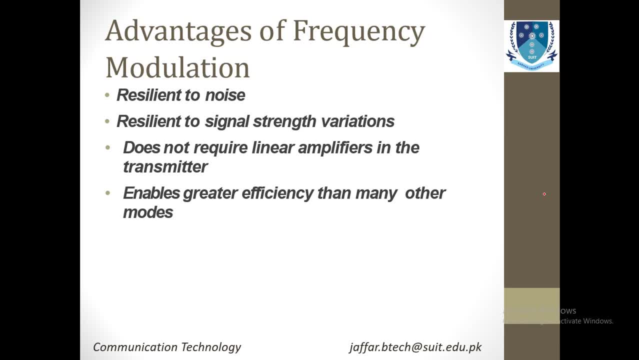 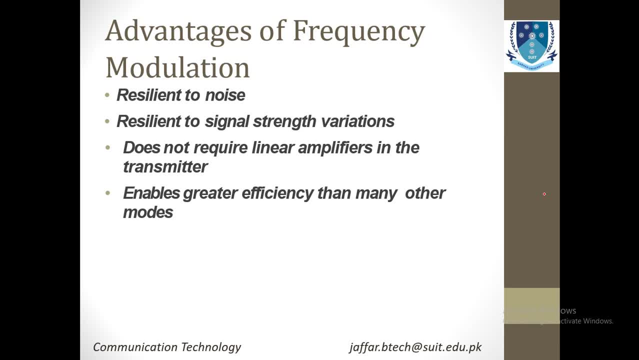 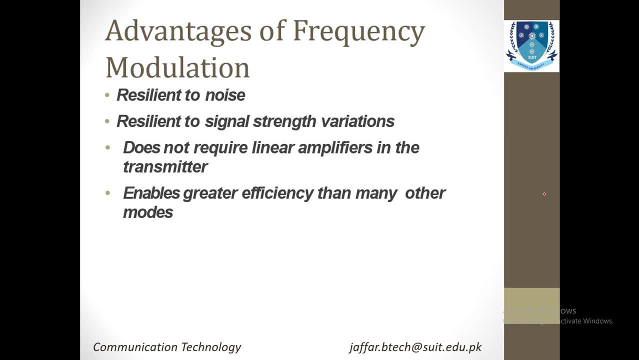 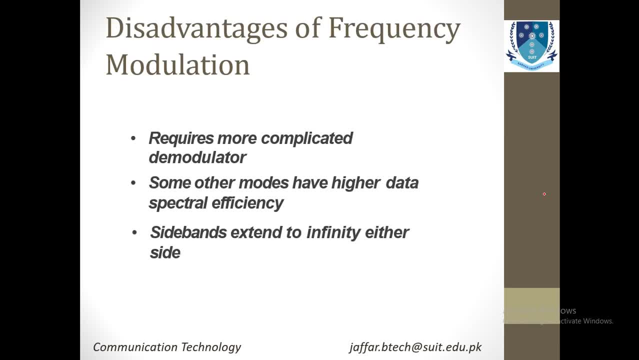 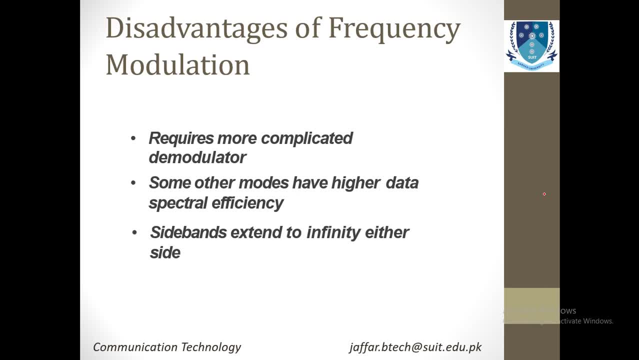 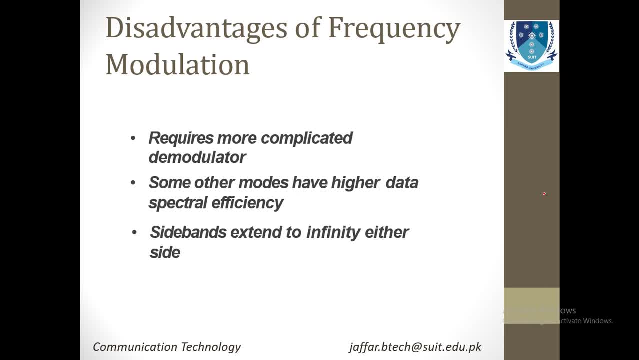 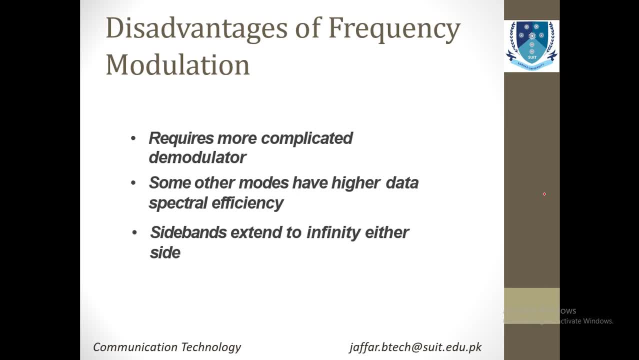 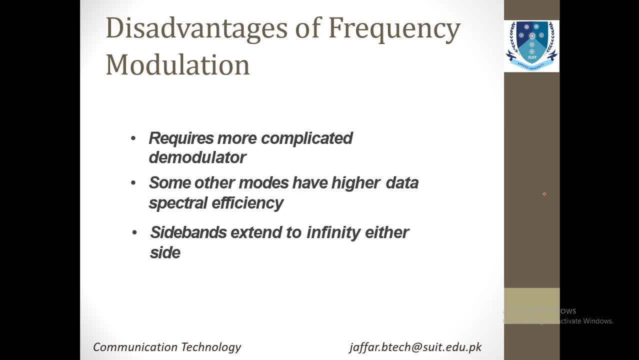